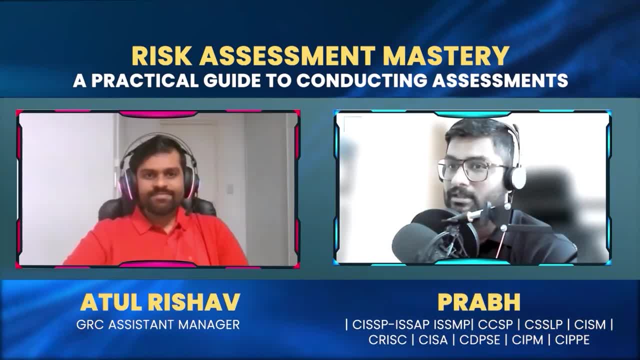 can you know a family member? it's a big thing. so, uh, you know. thanks, atul bhai, for coming out and taking on the time, that's all right. the session, that's all right. thank you so much for having me here and really privileged and honored to be speaking with you on record decision and probably 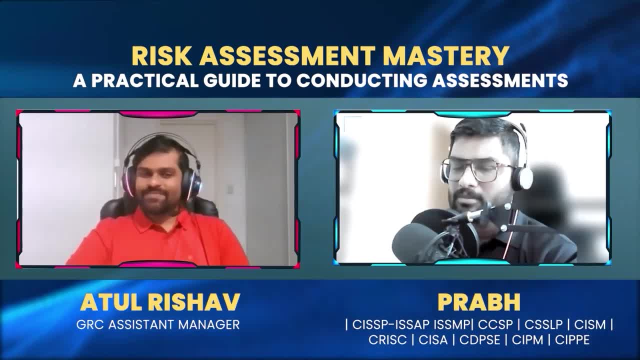 for life. so, yeah, thanks, thanks, atul bhai. and before we basically start the session, you know i always ask one question: how was the journey in grc? how was the journey in cyber? like how you started? if you can spend two minutes, three minutes on the area, yeah sure, that's all right. so probably, 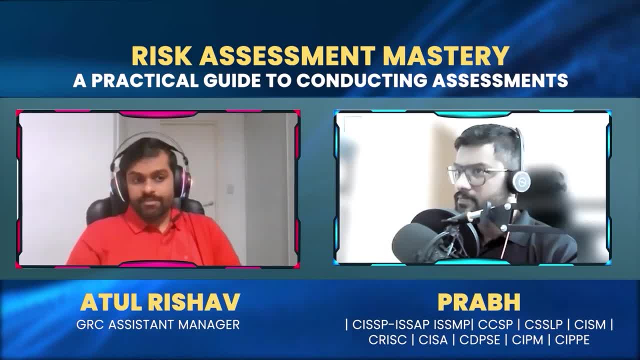 i'll start off with my educational background. so i'm an, i'm a bachelor's in electronics and communication and then i moved on to doing my master's in business administration, focused in oil and gas industry, which is, you know, very unique and which i'm not currently working in. 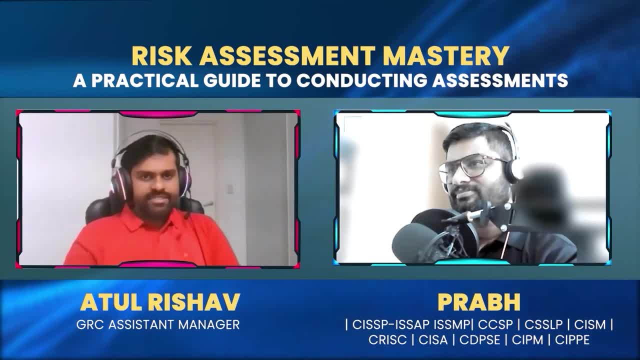 but i already i i always had this knack of, you know, being in technology, being a, you know, uh, being into technology, working on different technology, uh, technological tools and whatnot, and i really wanted to, you know, shape my career into any of the technology domain. i was not so focused on cyber security, to be very frank. i really wanted. 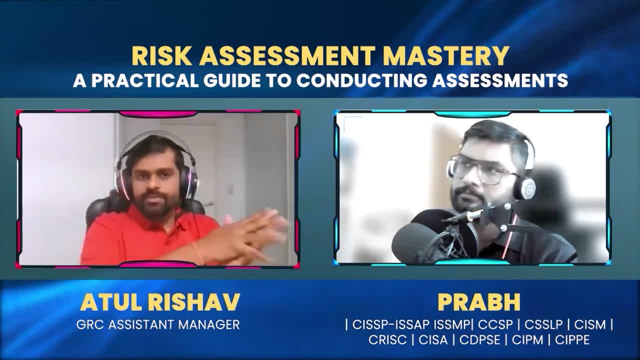 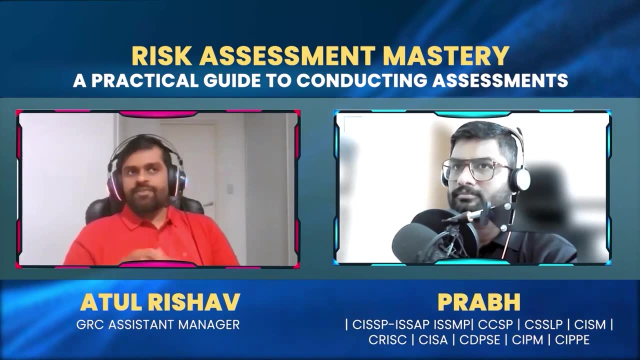 but as i mean, however, i really wanted to be into technology domain, right? so, um, when i started, when i completed my mba, i started off with these two startups back in hyderabad and punya respectively. i was working in research domain and, frankly, it's not about it, was not? 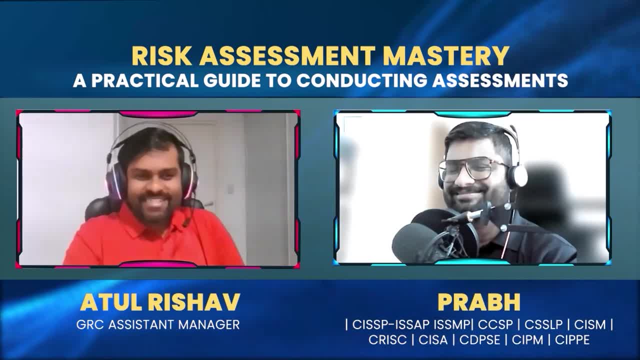 about the industry, but it was basically me who was not really, instead, interested into research and i really wanted to move out and do something of you know, make something out of me- or myself, for that matter, right. so i got connected, yeah, and then i got connected with a very old friend of mine. 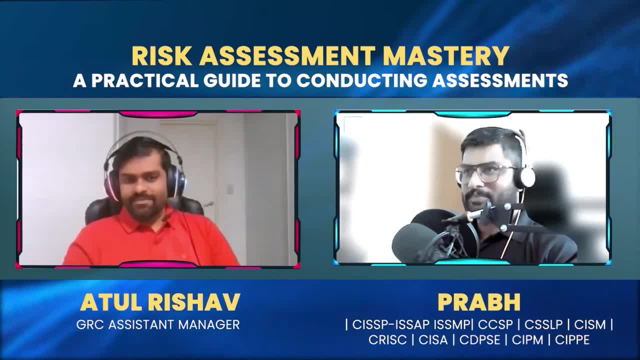 and he. so i'd say he. he's been friends for like 22 years and at the time he was working with ey. so i asked him: you know, could you please refer me? i'm ready to start from scratch. i'm ready to take a call and i'm ready to take a call. and i'm ready to take a call and i'm ready to take a call. 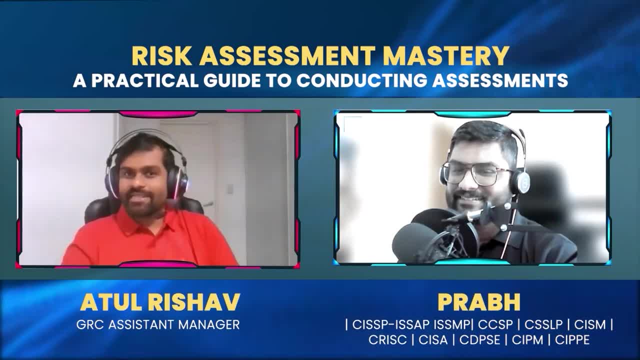 but i really want to get into something that's meaningful to me and i can shape my career into. that's, that's great, that's excellent, that's a great story coming from electric and today i know- see, i don't want to discuss another story, but i got to know today, but that is, that shows the quality and 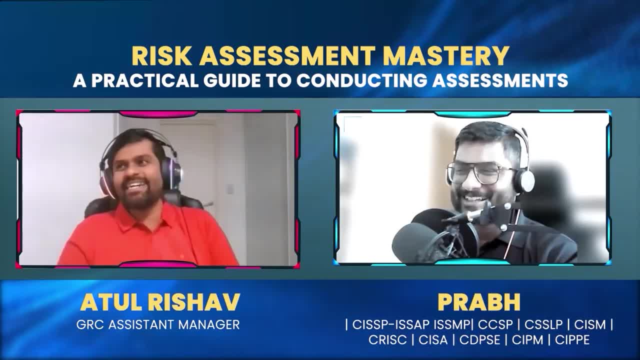 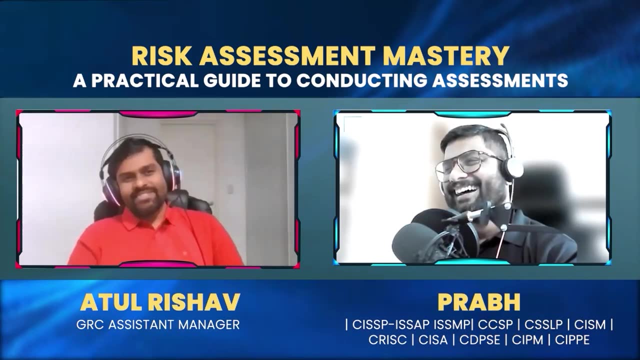 great characteristics of a good teacher. but let's let it keep it private. we'll discuss in another session. yeah, that's, that's right. that's right. that probably will polish that story and push it in some other session. we can, we can also bring the testimonial. absolutely, i'm happy to, and today we are here for what? what is special? 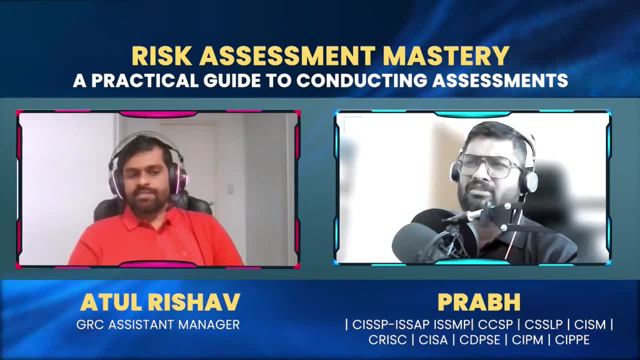 so we are here to understand the risk management. now, everyone there's a lot of videos other than risk management. what is special in this? so the special part in the risk management, is that, even if there are numerous materials out there into the market- you know youtube slide share- 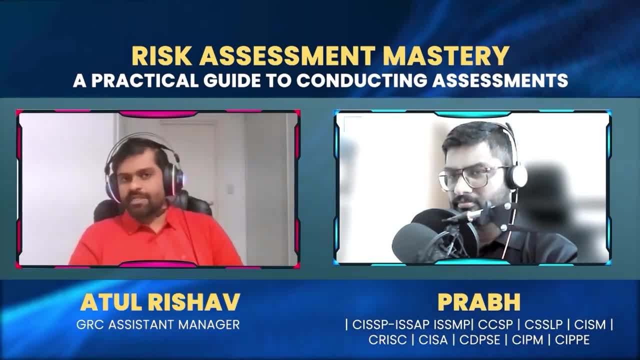 on and whatnot. you know- we, everyone knows that- what risk management did. but the fine line comes that how do you actually implement it? do you understand your risk? do you understand your business? do you understand how the business and risk relates to each other and how are you able to? 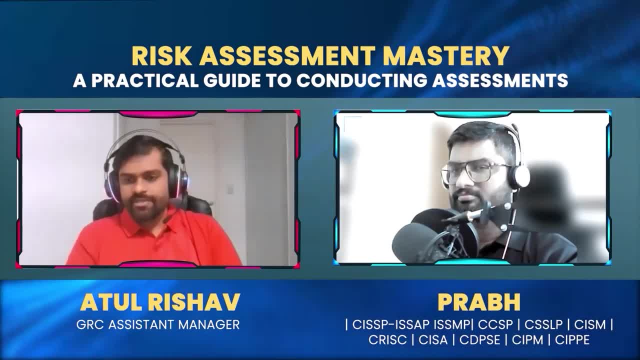 you know, probably mitigate it. what are the different criterias, what are the different techniques that you should be taking this, this, not always. you know you're going out in the market and you're saying that you know i don't have a, I don't have a PAM solution within my organization. 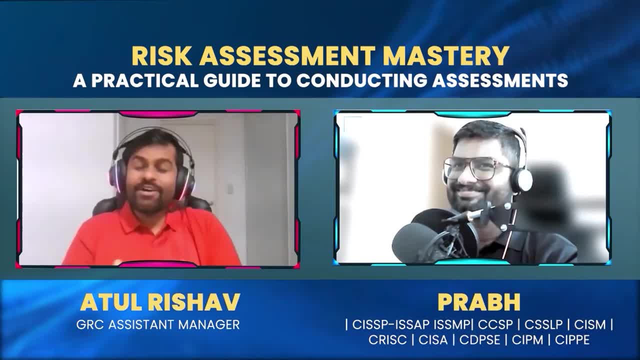 Let's just spend $100,000 and implement a PAM tool, right? That's not how it works. That's not how you should be mitigating the risks. There's a proper process. There's a proper visibility to the organizations. 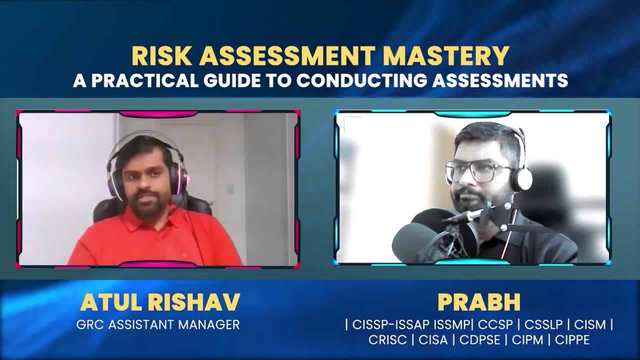 executives, boards and whatnot, right. So in today's session we would be covering that: how risk management actually works, not from a theoretical perspective but from a practical perspective, having worked with different industries myself into different markets, right. 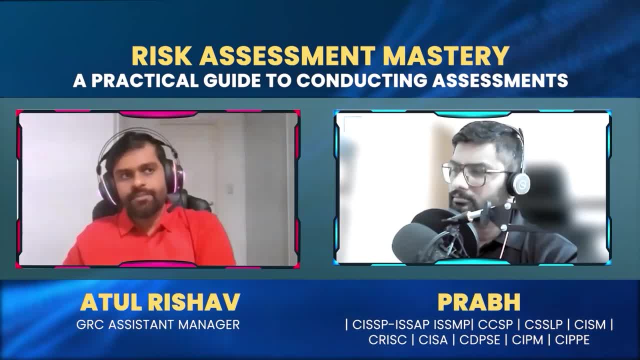 And with different complexities and size of the company. I do, and I'll not say that probably I'm entirely expert as of today, but I would say that I've had fair hands-on and understands how a business works and how risk management is an integral part of the business. 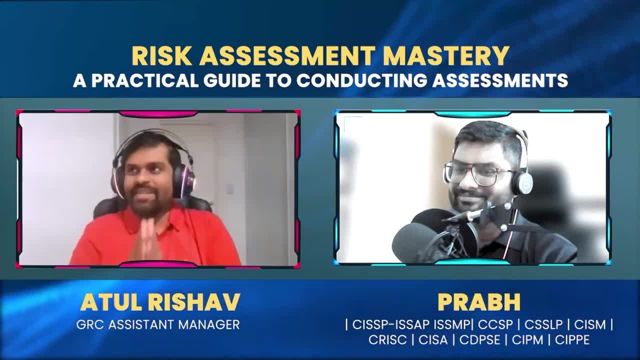 And cybersecurity is not about coding. I've been preaching this since I have started my career. It's not about coding, It's not about hacking, It's not about the green screen that we use. We all see the movies and we get into the organization. 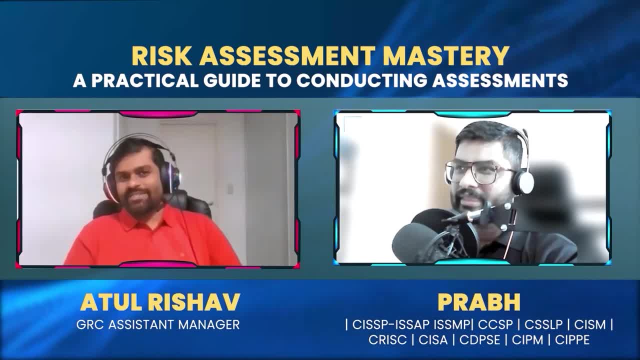 you know, just like that, It's not how it works, right? So there's this plethora of things that we need to consider. You know, it's about people, It's about process, It's about technology, right? The amalgamation of these three characteristics. 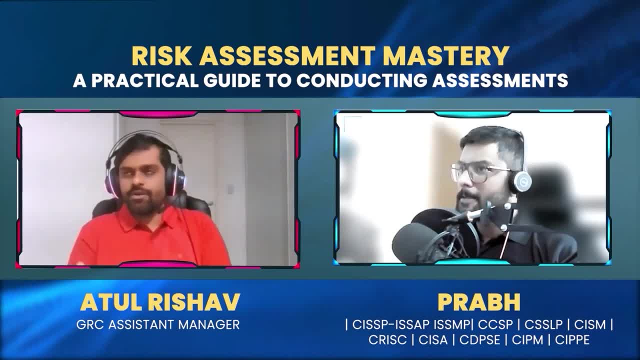 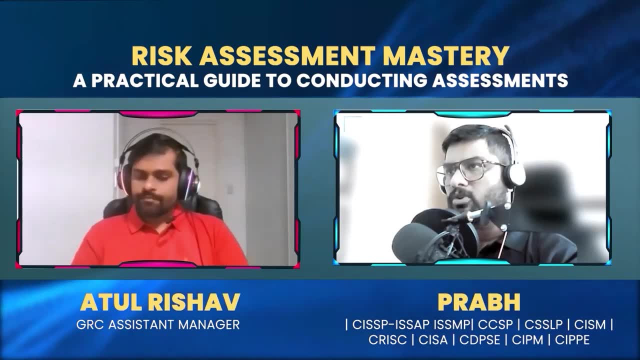 and the aspect makes the cybersecurity industry as a whole. you might say So yeah. So what I'm understanding from this particular session, it will be more like a hands-on where you know quickly drive to risk assessment. So, team, please do watch this video. in the last 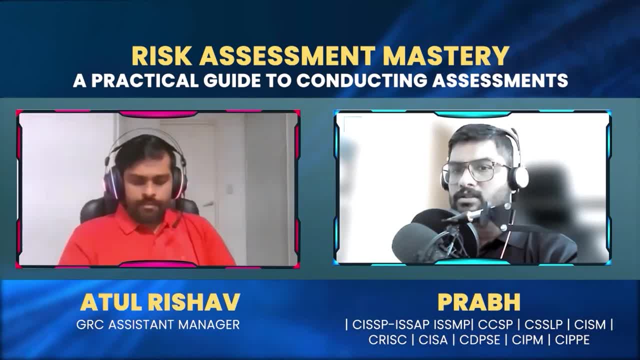 because, trust me, before we record the sessions and all that, we did a lot of homeworks. Atul did a lot of homework to make sure we can able to- he can able to- create a great value to this time and all that. 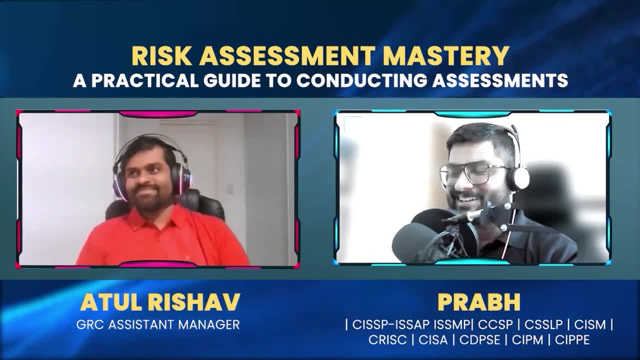 Trust me, I've seen his template and it is literally. it blew my mind because we have this way of understanding the risk. so, which is basically a great thing, Atul. So, without wasting your time, you know, Atul. 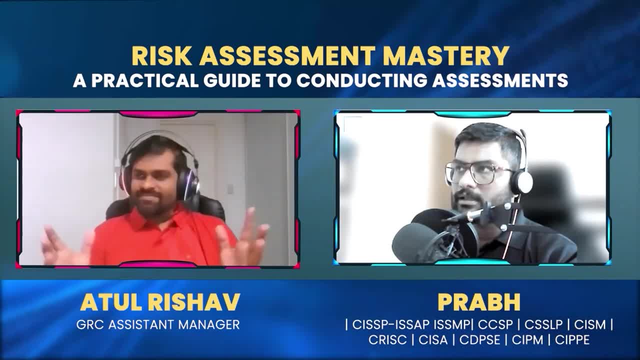 I'm giving you the whole strides so by that you can able to claim you can share your screen. Just give me a second Sure, Here you go. All right, So I'll start off with giving a glimpse of a risk assessment template. 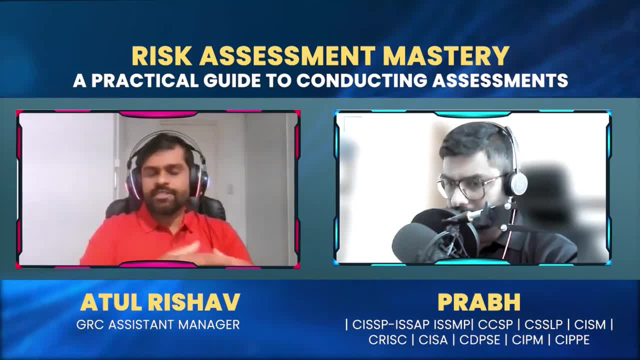 you know how it looks like, and then we'll deep dive into different terminologies that we use with risk assessment template so that it makes sense, And then we will talk about the entire world of risk management and how it works. But I can say to everyone, while he showing the document, 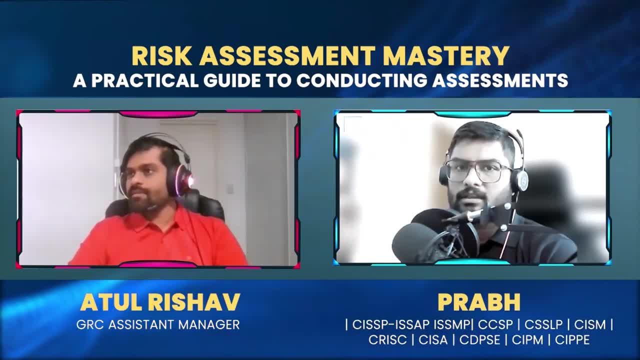 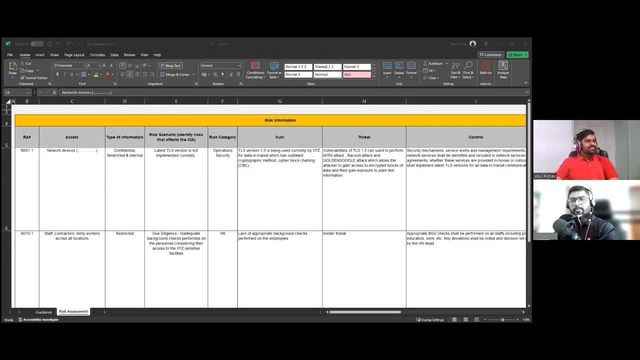 and all that, this video. after this, if your thought process doesn't get changed about risk, you change my name. And I will assure you one thing: after this video, even if you're preparing for GRC jobs and all that- 60% answers- you can able to get through this video. 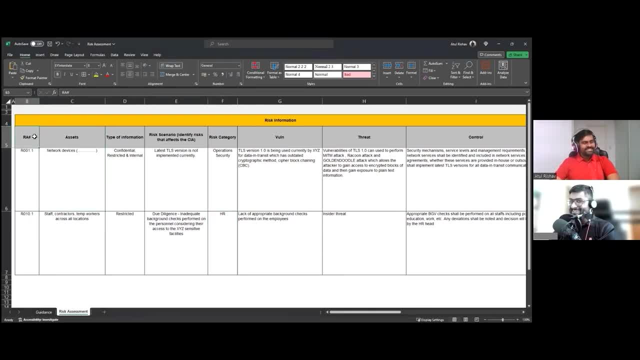 Trust me, I know this guy He because, before we record this session, that kind of a testimonial he shared and the experience train one person transitioning from the non-information security to GRC. I'm sure this guy will go to the next level. 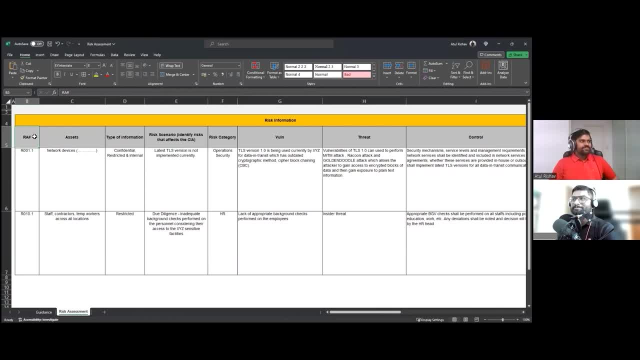 Thanks, Thank you. Yeah, thanks, bro. Thank you for thank you for the kind words. All right, So I hope my screen is visible. Yeah, yeah, All right, So I'll just give a glimpse and probably I'll just run you through. 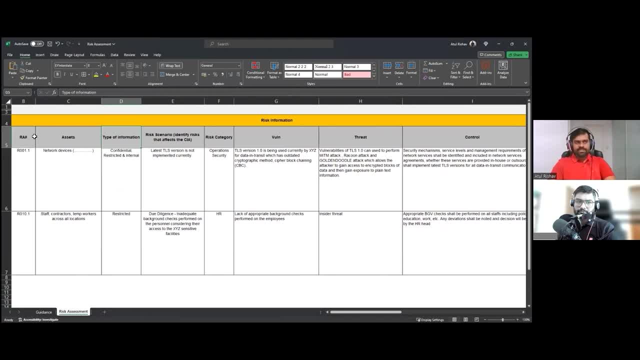 the terminologies that I would be using. Okay, So I'm using the standard risk assessment template And obviously it differs from company to company, But, however, at the same time, it will give you a fair idea that what information should be there in a risk assessment template or in a risk. 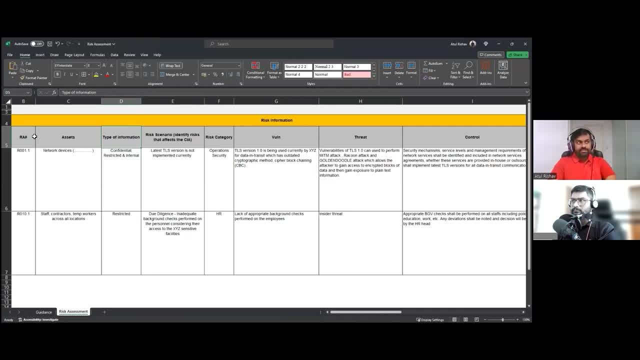 assessment process, to say the least. you could add whatever information you would like as for the business requirement, But these information are baselines. These needs to be there in a risk assessment. Okay, So, Yeah, right, uh, we have got type of information. what kind of information is? is that particular asset holding? 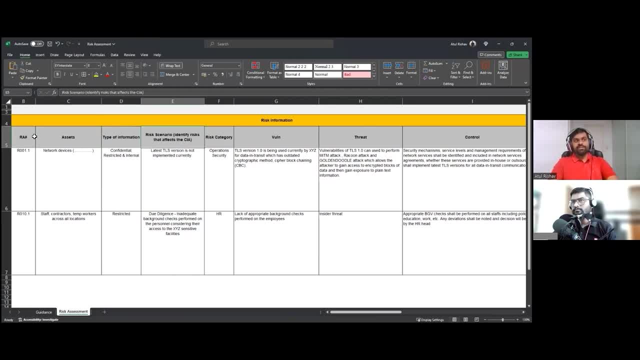 we have got risk scenarios. so risk scenarios is nothing but the known risk, known risks or known uh vulnerabilities. that's out there and we know that. this is there and we need to mitigate that. so this is, this is the risk scenario. we have got the risk category. we have got what kind of 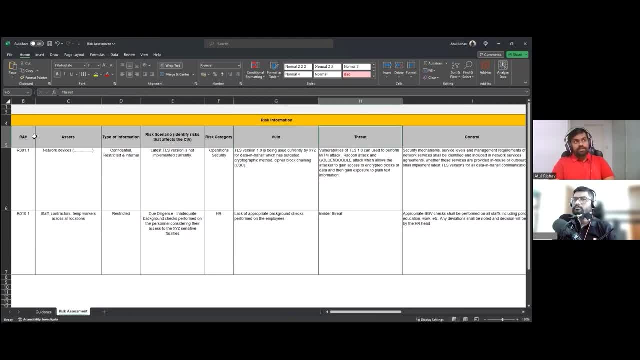 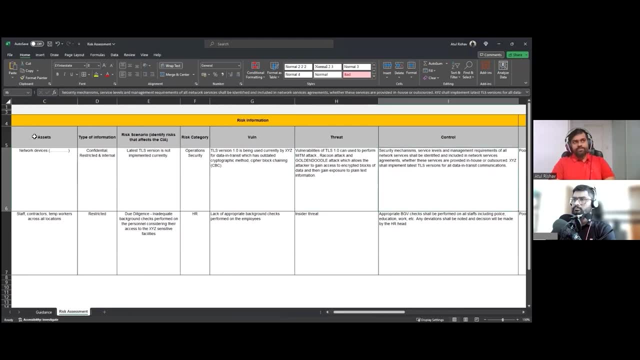 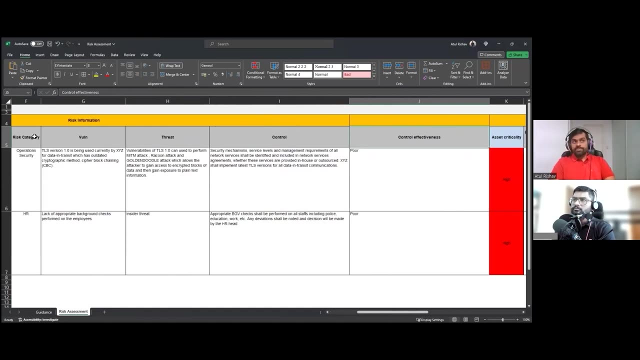 vulnerability relates to that risk. what is the threat? uh related to the vulnerability. what is the control that needs to be there so that it gets mitigated to an acceptable level? and we'll talk about that in in our later uh later in this video. uh, we have got control. 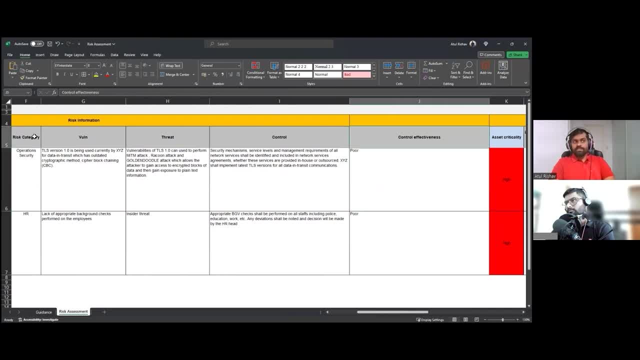 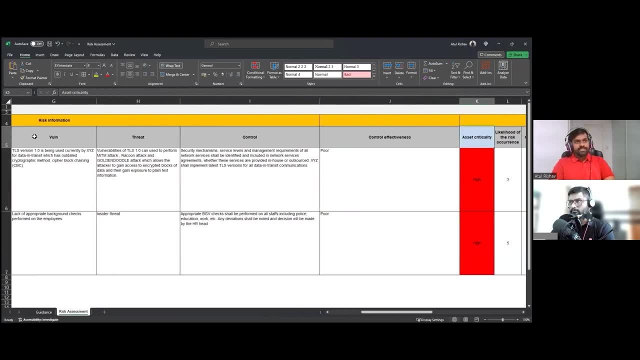 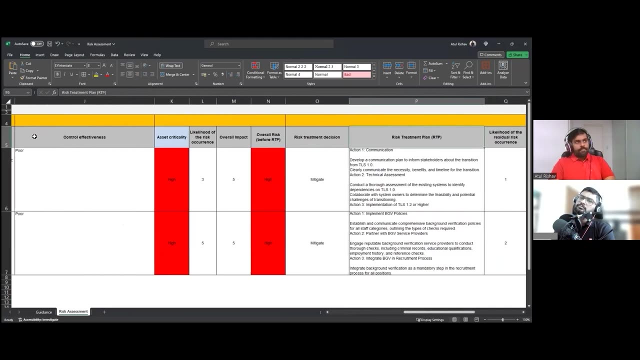 effectiveness. so, whether or not it is, uh, it is, it is achieving to its full potential, or is it poor right now? uh, what is the asset criticality? so when we see asset criticality, it is this asset. so network devices, staff contractors will speak about this. um, then we have got likelihood of the risk, we have got the overall impact of the risk on the business. 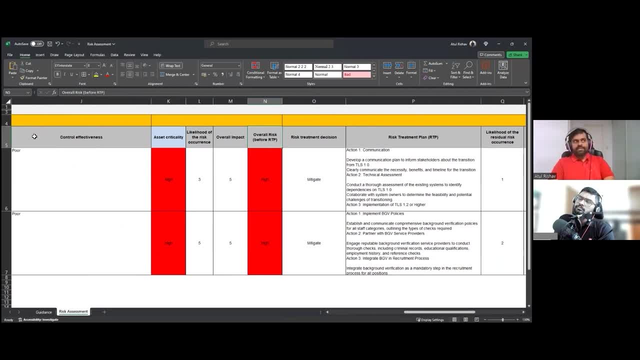 and then we have got the overall risk rating and this rating is before applying the control that we earlier showed right. so this should not be confused with the risk that, uh, that's there after applying the control. so, in other words, is the inherent risk that we that we speak about right? and then what is the risk treatment decision that we are gonna? 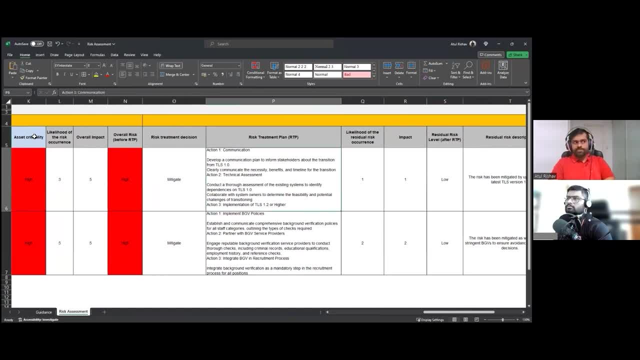 take right, uh, what is the plan that we are gonna do? so i think, uh, it's, it's, it's pretty long, but then, yeah, i'll deep dive into that and just praying to the customer for whom you are working, increasing his effort and increasing his work. i know i mean, that doesn't go well down the road. 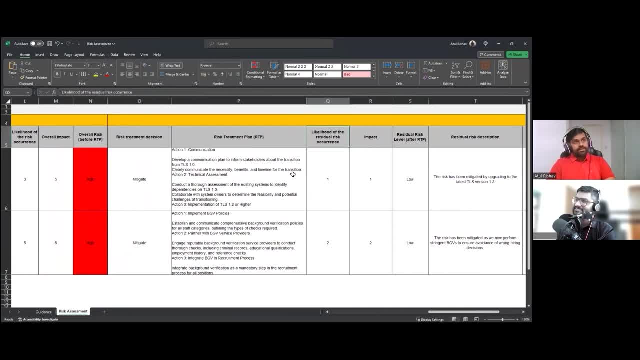 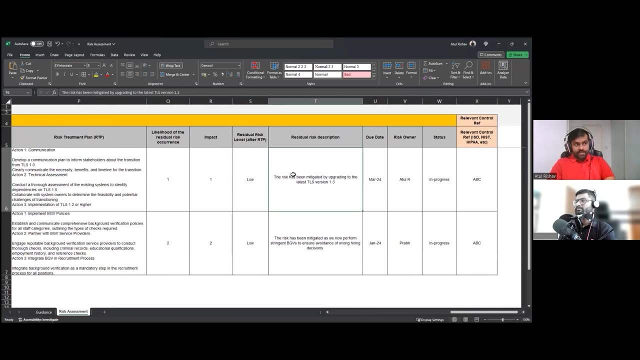 yeah, um, then we have got the likelihood, impact and risk again, but these three, but these three parameters that we talk about is after we apply the control and after we apply the risk treatment plan. um, furthermore, we have got the residual risk description, so whether or not the risk is, uh, below the 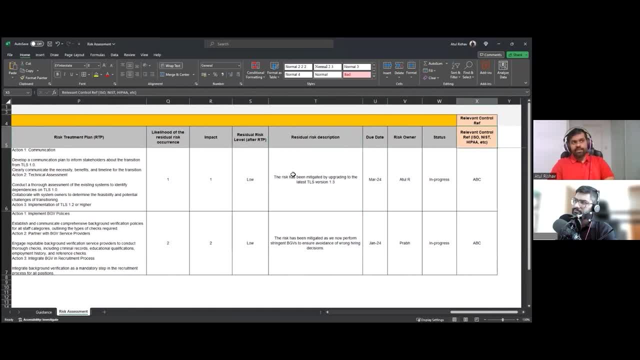 acceptable level? right, and what is that we are looking at? is it? what is the due date? who's the risk owner? probably have assigned you one and what's the? what is the status of the risk right now? and what's the? what relevant control does it maps back to? so, yep, so we have got iso, nist, hipaa and whatnot. 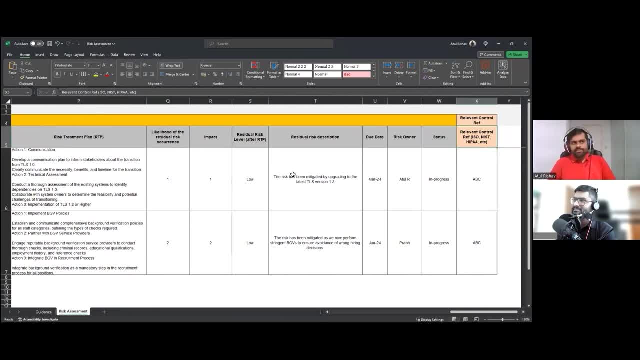 so we have numerous- you know, probably uncountable- cyber security standards out there, right, and whatever cyber security standard you are taking as a base for your organization, it's highly recommended- highly recommended- that you refer the exact control number or exact reference to each risk so that whenever you are going for an audit or internally as a 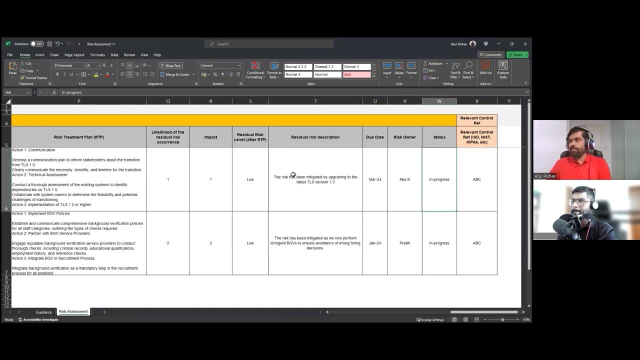 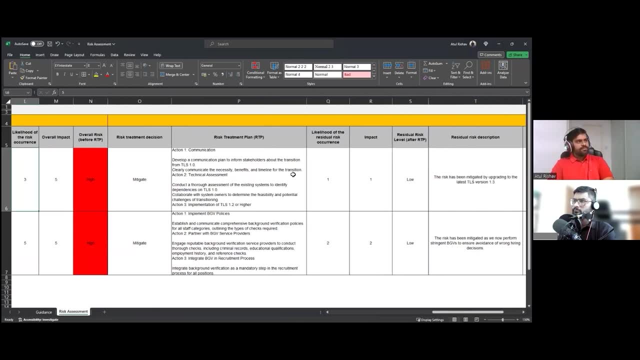 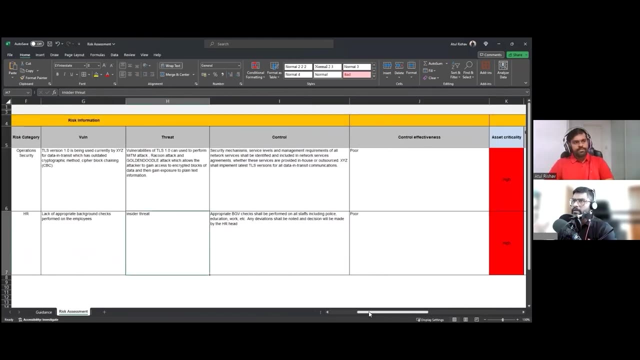 well, you have a proper visibility as to what control are we talking about, right, okay? and whether or not we are complying to the control as a whole, right? so this is a fair bit of- probably- glimpse on the risk assessment template, right? so, before we basically start this. so yeah, as you know, 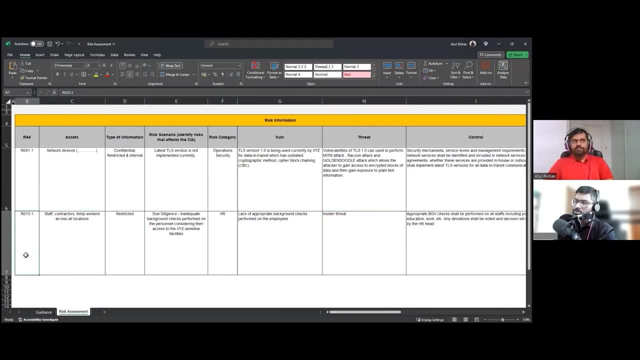 this video will be also viewed by the lot of people who are new to this topic. so is it okay? we can spend 10 minutes to understand about what is asset, what is threat, what is one absolutely risk, and then we can directly jump to this particular template. so, guys, we are going through. 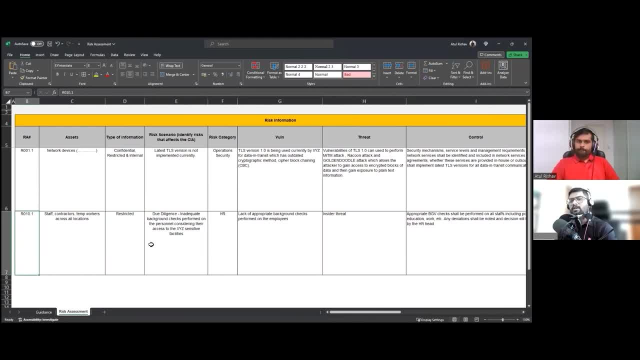 the basics first. so don't assume that, okay, we are the expert or you are the expert. let's start with the basics. you might get a new insight and then we'll come to this particular uh, this particular template, right? so? so anyone who's starting off in grc, cyber security and- and look, i mean it's not- 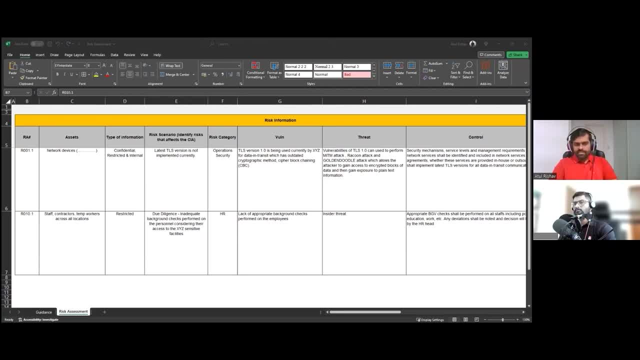 about being into grc. it's more like the risk assessment methodology or the risk management framework should be known by everyone, any technical or non-technical person working in the cyber security. but because we, everyone and all of us play a part to reduce the risk as much as possible. right, and i always preach this and i always say: 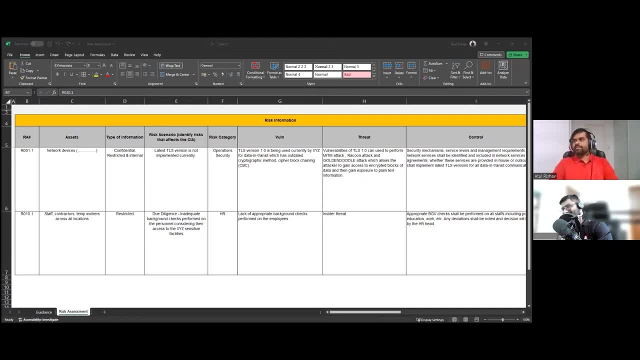 this. you cannot reduce your risk to a hundred percent level, right? you cannot. you can never, ever. there will always be a risk for you to get hacked and there will be always a risk for you to get compromised. the best you could do is to make it mitigate it to a level so that you are comfortable. 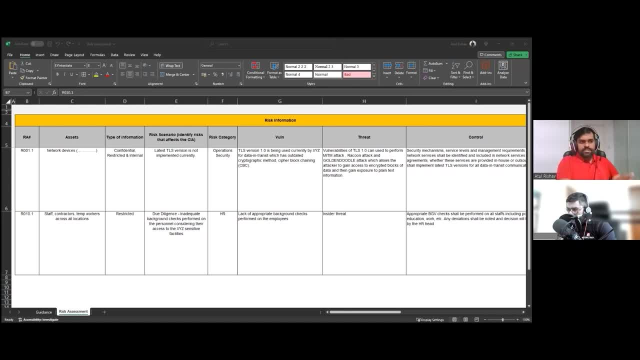 even if you get hacked, the level of data or the kind of data that gets compromised, it's not so important or it will not have a material impact on your organization. so that's that's, that's, that's the, that's the overall. you know, probably i'd say the overall uh agenda of the risk management. 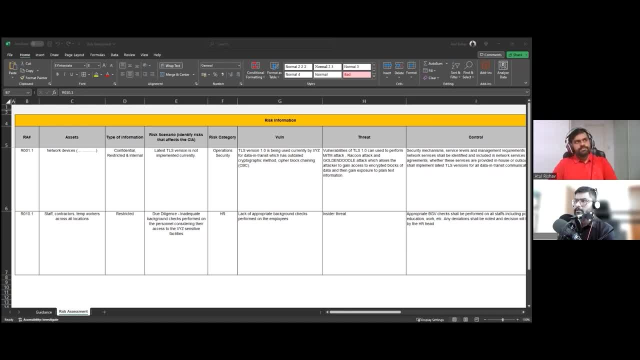 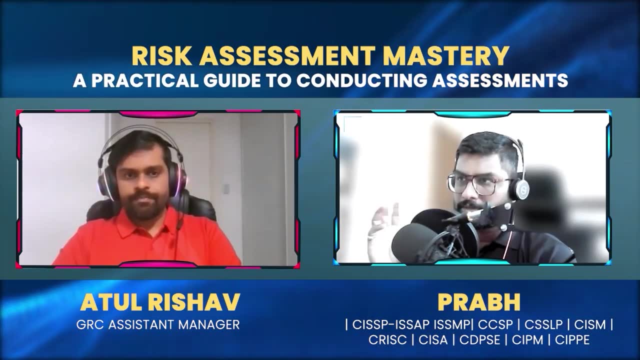 framework that's being used across the organization so great. so i'm saying that when you're talking about the basics, right, well, what is right? what is threat? what is vulnerability? what is threat? what is right? you're sharing me that particular content, right? so can you just share? that's right, yeah. 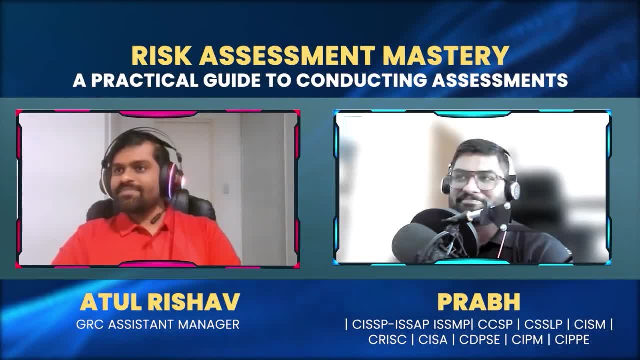 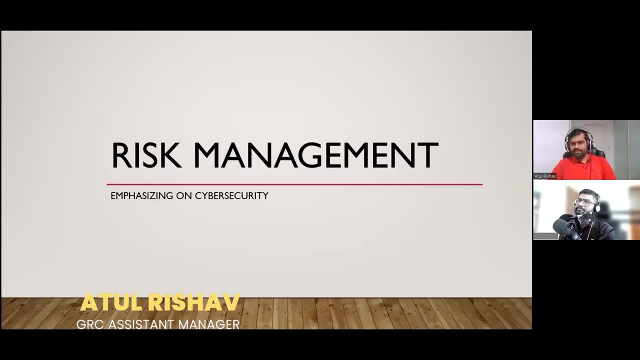 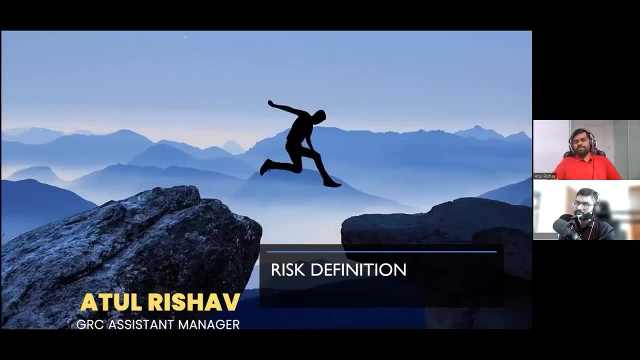 yeah, yeah, yeah, i'm saying too much, i'm in too much demand. oh, i hope the. yeah, it's visible, all right, perfect, so all right. so let's get started with the definition of risk. so we did speak about, or we did have a glance on, the risk, on likelihood, on threats. 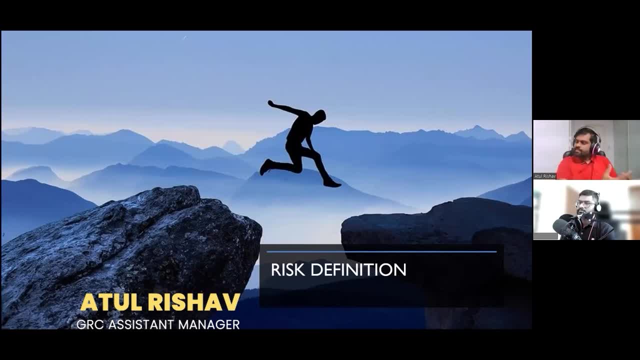 on the risk treatment plan, on the kind of mitigation strategy that we are going to adopt and whatnot. right, so we'll just i'll just touch upon basic definitions. i'm sure this plethora of information out there in the, in the market, and you know people can go out and uh deep. 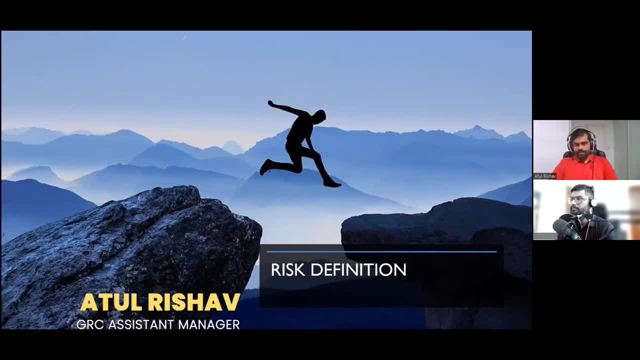 dive into each of these topics, but i'll try to have a have a basics covered as much as possible. so, what is risk? risk is the possibility of something occurring that could have an impact, right? so all right, let's take an example. i have a glass of water, right? what is the risk? or, probably there's. 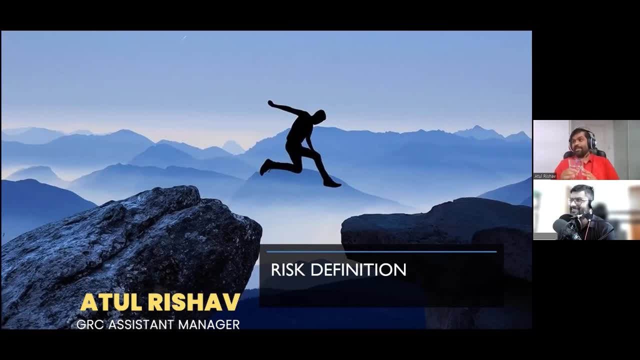 a risk that this glass might fell down off my hand and it will break. and there's this another risk that i'll step onto the broken glass and i'll hurt my leg, right. so this is the risk that we are talking about, right, so risk is as a whole. it does not only release to cyber security, but it relates. 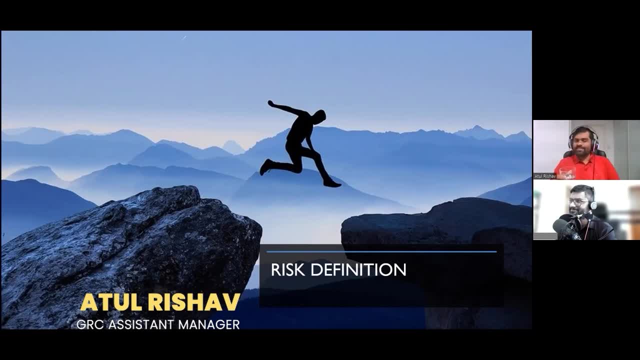 up to our own personal life. if you are crossing a road, what is the risk of you getting hit right or a vehicle hitting you right? what is the risk? you probably, at least in australia, you don't get hit as much as you get in india, but that's it. there is always a risk, right. so this is the risk that 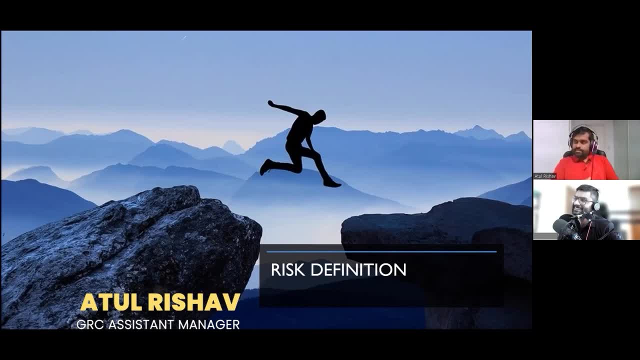 we talk about it is the occurrence of an activity or an unforeseen event that might have an impact on you which is not in your favor, right? so this is the risk that we talk about. what is the risk if that in a glass we have a beer? well, that's not a risk. 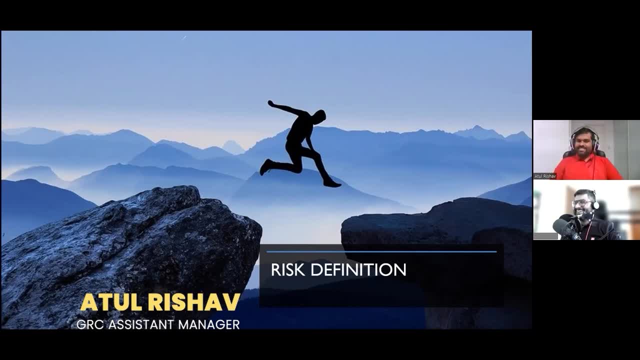 that's good times. that really we are talking about, isn't it? we might have some threats. yeah, i mean, you know, getting passed by my wife, that's, that's a risk. that's a risk. it's all about what kind of a control you have. you know how you basically present yourself during that time. you 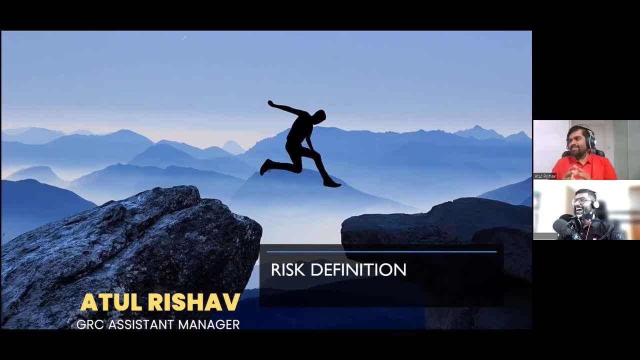 know. no one can get recognized. you are. there's only one control in this situation. i don't get back to home in that night and impact is right, then you might lose the house, i'm very certain about it. i'm very certain about it. but but but it is a risk, it's not an incident. 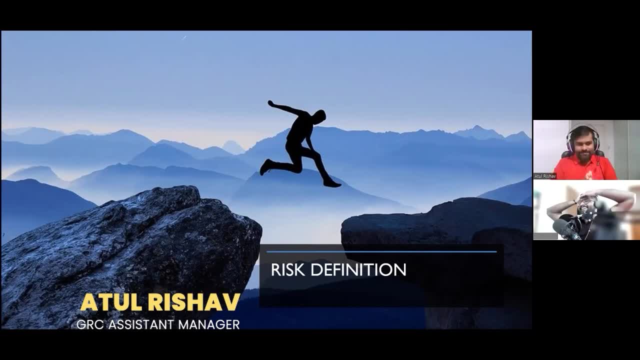 if it happens, it's not an incident. yeah, it's not an incident, it's a risk, but i mean in in that's, in that scenario, probably convert, get converting from a risk to an incident is highly likely. that's how we need the controls, right, all right, okay. so moving on, what's our vulnerability team? so a vulnerability? 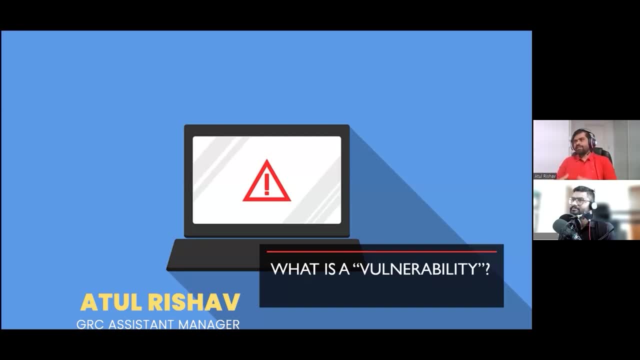 team is nothing but a weakness, right? so it's an inherent weakness within the system or within anything that's a vulnerability. so probably, i'll take a technical example here, maybe. so, let's say, as an organization, i'm using windows 2012 r2, right? i'm hosting all my data there, but i cannot upgrade. 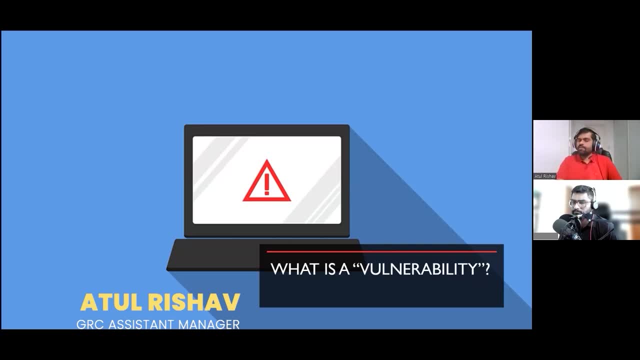 because the the application that i'm running on that particular server does not support the latest version of the windows server. i can't do anything about it, right? however, at the same time, we all know that windows 2012 r2 is vulnerable or susceptible to certain attacks. 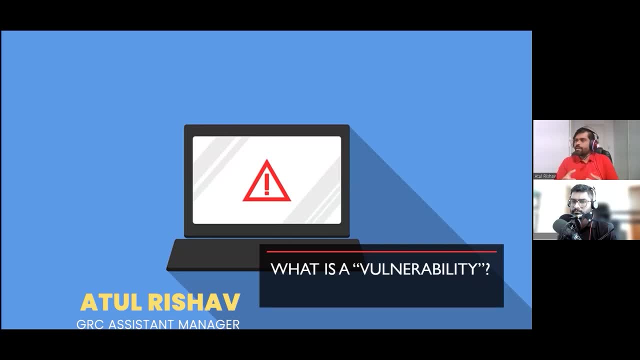 right, rdp, exploitation, rc and whatnot, right? so we know that the availability is present in there. so vulnerability is nothing but a weakness which is already present and known, probably by the threat actors or by the organization. so that's, that's a vulnerability that we are speaking about. okay, right. 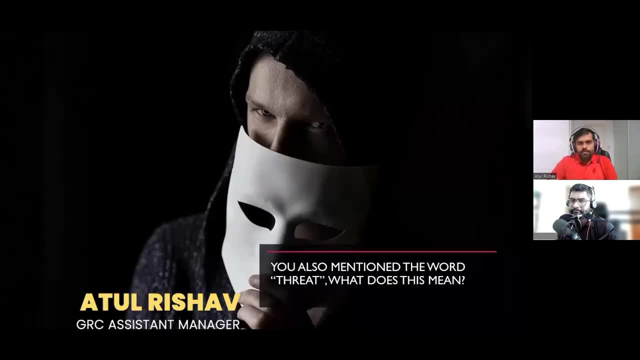 let's move on to the next one. so i didn't mention about threat. so what is a threat? a threat is nothing but how you exploit that vulnerability and use it to your- you know, uh, uh, your own, uh, interest, right? so a threat could be exploiting the windows 2012 r2 server and and getting into 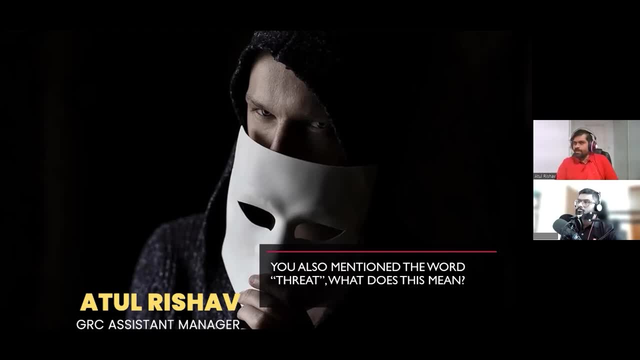 getting into the server and exfiltrating all the data that that tools right. so that's a threat. and then we know that that threat, uh that vulnerability, can be exploited. that's the threat. and a threat actor is nothing but a person, an organization, a process, an application. who is 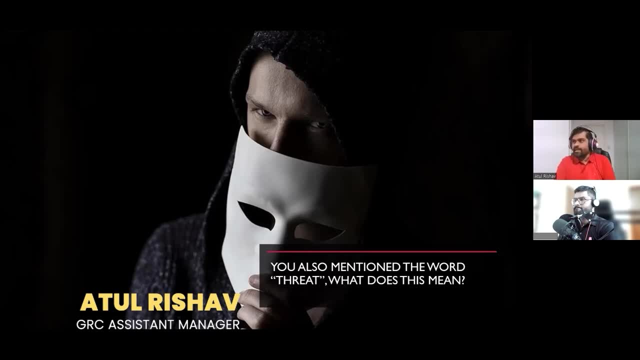 conducting that phenomena. who's who's doing, who is exactly doing that right? so that's and that's a threat actor that we're talking about. a threat actor could be an insider inside a threat actor, right? someone within the company, you know. 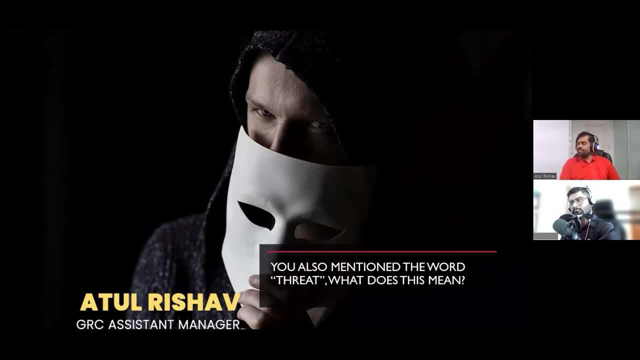 the information to uh, to a malicious actor, stating that you know we have a data center here, these are the servers that we are using and whatnot? right, um could be hackers who are who are attacking from from external perimeter, getting infiltrating into the, into the inside network, and and whatnot. 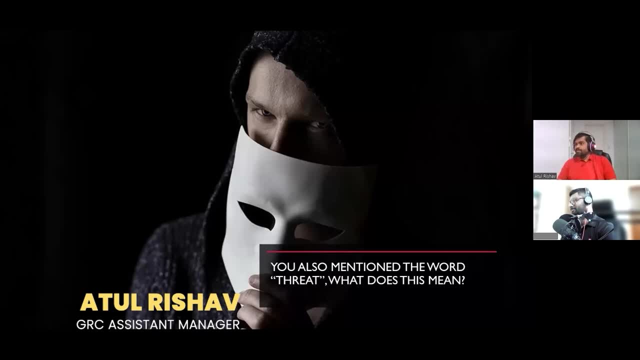 right, it could be an organized crime, right. ransomware gangs- right, they are threat actors, they are exploiting an unknown vulnerability into the system, right. so that's that's. that's. that's that's a threat that we are talking about all righty. so let's talk about likelihood. 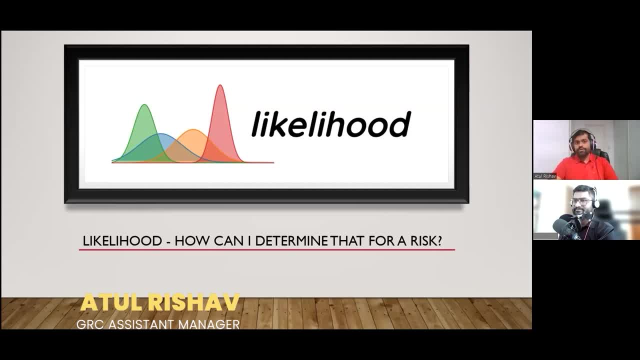 likelihood is, is something that you know: what to what frequency, or what is what is the what is the time, i would say time frame, that's not the right word, probably, um. so this is something that you know to what extent this vulnerability can be exploited. so say that a windows 2012 r2 server. 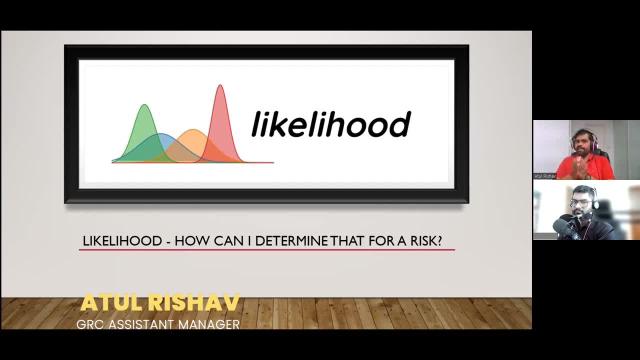 it's highly likely that anyone using it can or are susceptible to the attack by the threat vectors that we spoke about. right, it's highly likely. however, as opposed to someone using windows 10 or windows 2019 server or windows 20- 2016 server, they will have a very less probability or probably. 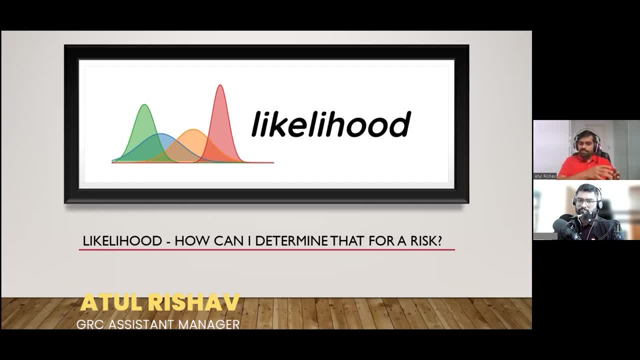 less likelihood of them getting attacked because uh, those, those servers or those machines are are still uh under under microsoft patching. you know uh patching scheme and they- microsoft does releases a lot of patches for them, right? so they are still there. so the likelihood of them getting attacked. 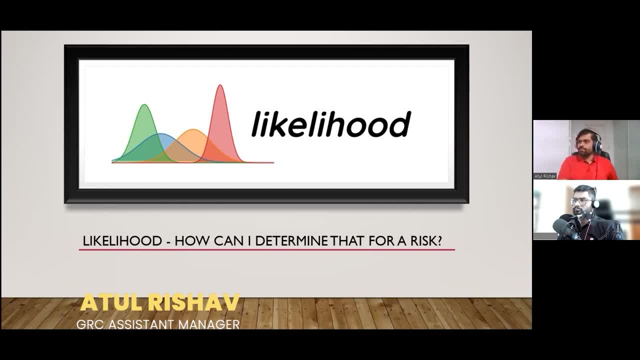 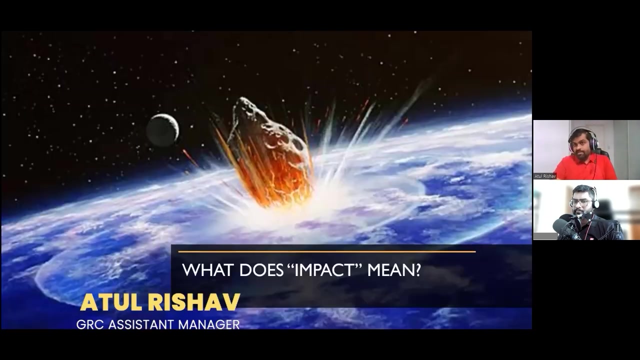 would be highly low as opposed to a windows 2012 r2 server. right, so likelihood is nothing but the possibility or a probability of a threat actor or a threat actually exploiting the vulnerability. so, yeah, that's sad. okay, let's move on to the next one. yeah, this, this is something really important. 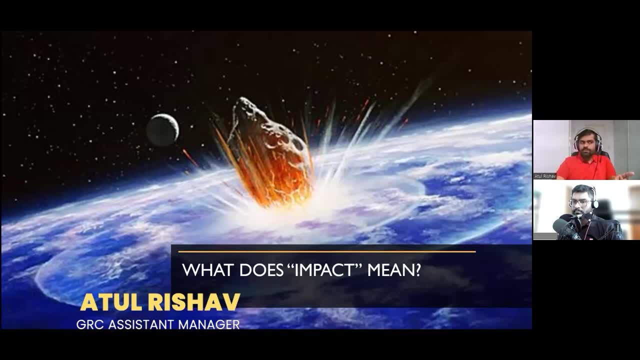 to the business. this is what business exactly looks for. what is the impact? right, if my system gets compromised tomorrow? what is the impact? that we are looking at? and it is really subjective, you know. so, uh, with smbs that i have worked with in the past, uh, they usually don't go for quantity. native method. they usually go for a qualitative method. however, with the big organizations, with the fortune companies that i have worked with previously, i mean as a client- so they actually go for a for a quantitative method. so, for instance, say that i have got 100 laptops right, hundred. 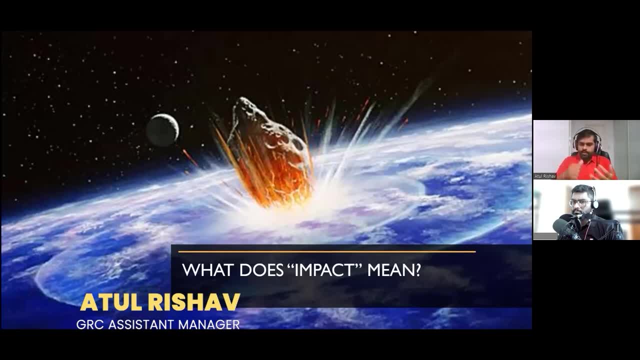 laptops being used by critical business users, including board members, including executives, including it team, including someone who is having a privileged access or escalated access or a right. i've got hundred, hundred systems with me, right, each system costs me a thousand dollars. right now. those thousand dollars multiplied by hundred laptops becomes my exposure, right? 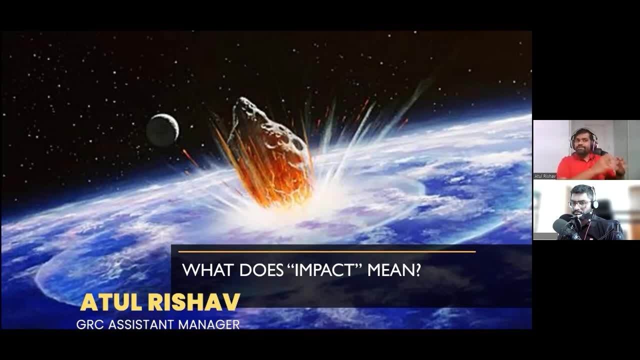 if something goes south, this is the actual asset value that's being compromised. that's being compromised and that's something we are looking at. and we are still not taking the data in account, the data it holds right. the data could be more valuable than that right, so say that you know, uh. 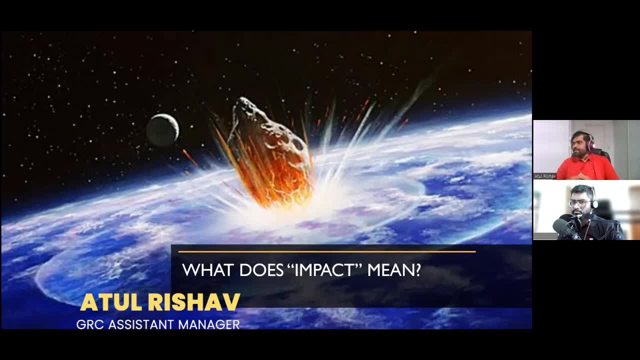 all those systems hold some kind of sensitive data- pii data, psi data, phi data, for that matter- right, they hold some kind of the some, some of the other data with them, right? and one of the reasons why people are going on cloud, one of those reasons why, uh, people use vdis and whatnot just to make 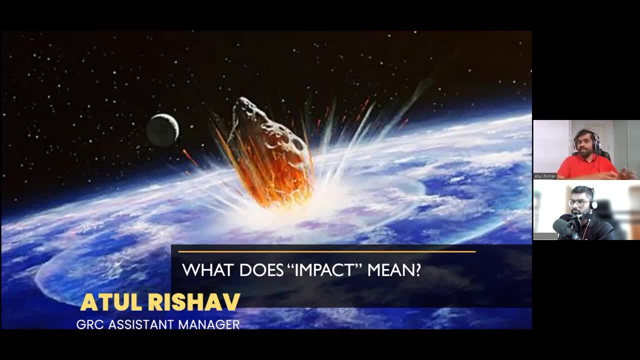 sure that these sensitive data are being isolated somewhere else and not located on your laptop, so that, even if your laptop gets compromised, the threat actor doesn't have access to your, to your system. right? not all the times, bitlocker will save you, and that's the thing. that's the reality, so so, that's, that's the kind. 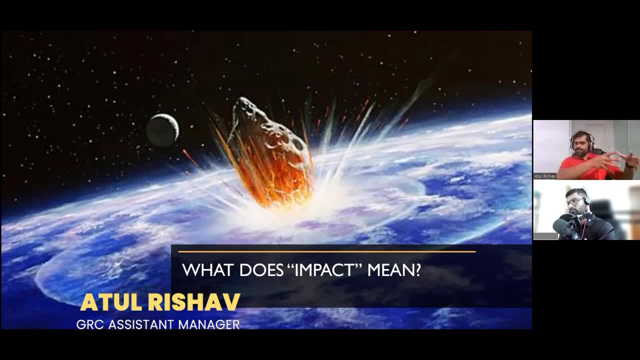 of impact that we are looking at. so there are two, two aspects to it. so the first aspect is the monetary impact, right, and the second- second second aspect is your reputational impact, right, if you, if you, get hacked tomorrow, right, if your portal gets hacked? i mean, we all heard octa breach, not 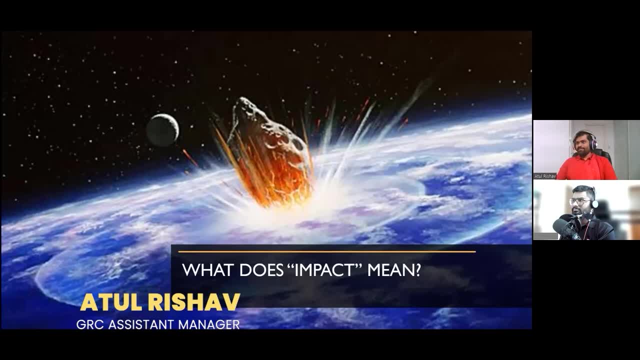 once, not twice, but they got these thrice right. and what, what reputation now it holds in the market. they lost a lot of a lot of customers. so for them, the, the, the reputational impact, trying the financial impact right, they could always earn back the money that they have lost during the ransomware attack or 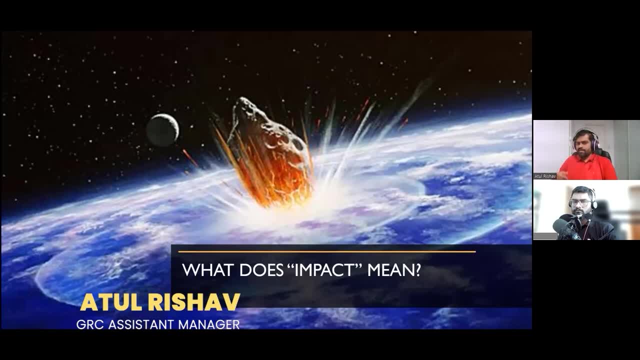 during, during. whatnot right for patching for operational, operational stops and bringing back the systems, you know. so all the operational costs that we are talking about, right, they can always earn back that money, uh, in the next five years and seven years, right, but the reputation that they 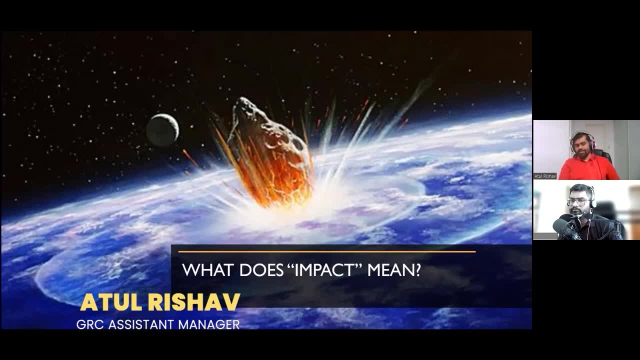 have lost, I'm not sure how they are going to be able to recover, right. it's really difficult, right, and it's same case, the same cases. I mean there are numerous cases across the world, so it's not only octa, it's across, I mean in India, in Australia, in some of the markets that I'm currently working in. 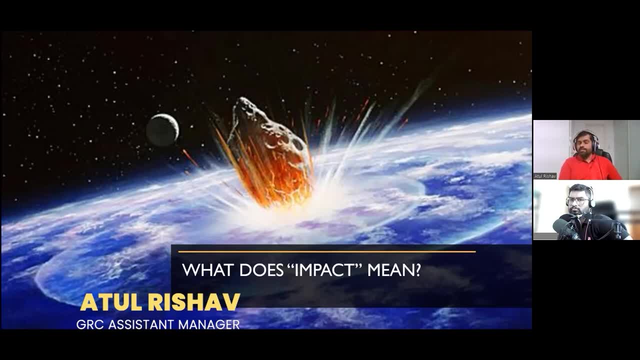 if the company is getting breached, it's not and it's not the financial impact that they look for, the impact that the board or the executives are really concerned of, because once the reputation is gone, it's really hard to win back the client again for them, right? and that's where the 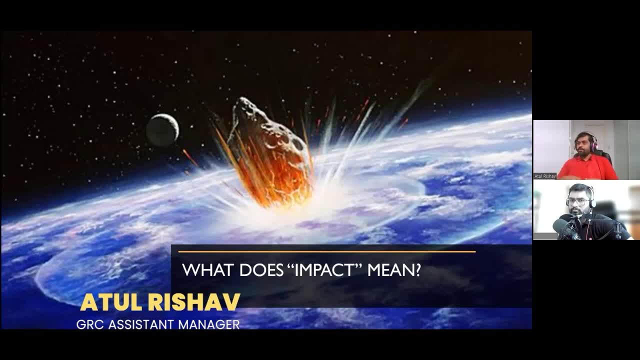 competition increases and that's where it's really important to know that. what your risks are right, what, what are the threats that you are looking at? obviously, you will not be knowing about any zero date, and that's- and that maps back to my previous statement- that you cannot and never, ever reduce a. 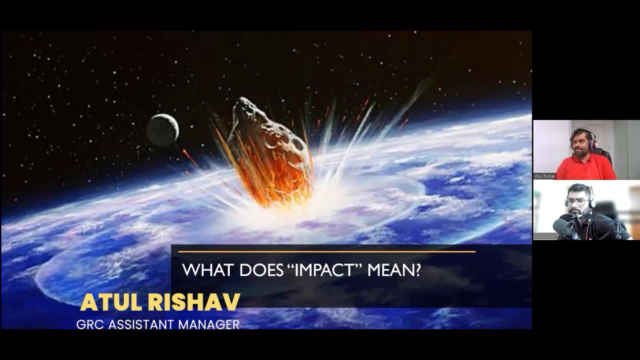 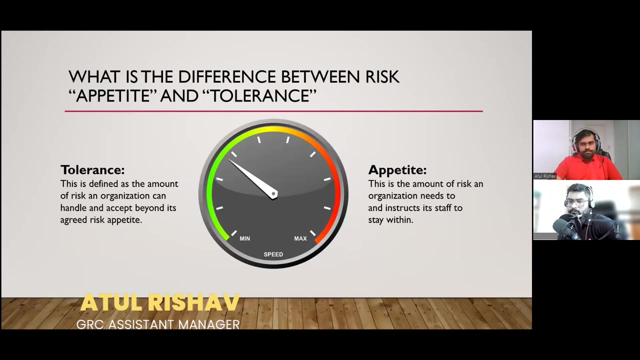 risk by 100. there will always be some, some or the other risk, but the best you could do is identify all the known risks which is applicable to your business and work on it. I agree with that, I agree. so the next one is, uh, risk appetite and risk tolerance, and oftentimes I've seen that these 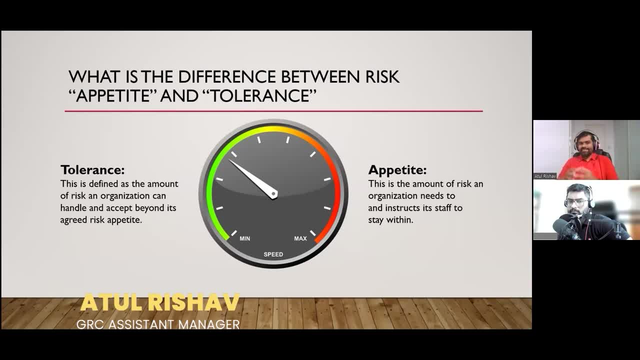 two terms are interchangeably used as a same definition, which is not and to be very frank- and I'm guilty of that- even I used to think that: a risk tolerance and a risk appetite. when I started off my career, I really used to think that we started the risk appetite. 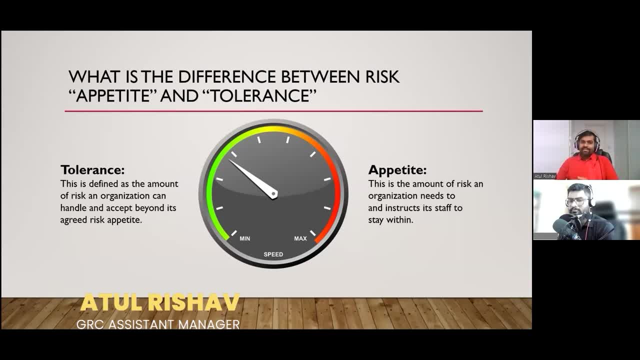 are the same thing, however, but it's not right. a risk appetite is something that I define, that this is, this is the ideal appetite that I'm looking at. I should not be going above that, right, so say that if I say, all right, let's take glass of water, yeah, so my risk appetite is that. 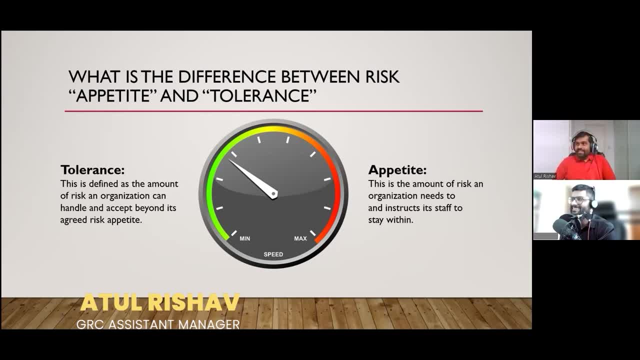 this class, this class I. I cannot raise this class to here, right, if I go anywhere above here, there's a, there's a high chance that I'll drop this class and I lose my balance. so the ideal, the ideal space or that, the ideal height that I'm looking at is this or below this. so this becomes my 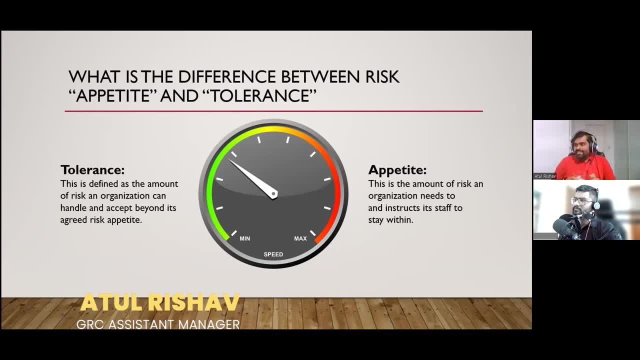 risk appetite. however, my risk tolerance is something that I take a buffer. I I know from you know from experience, or you say emotional intelligence, or you know any word. you could probably think of any single word that you could think of. I know that even if my risk appetite is this, I'm going to raise my glass. 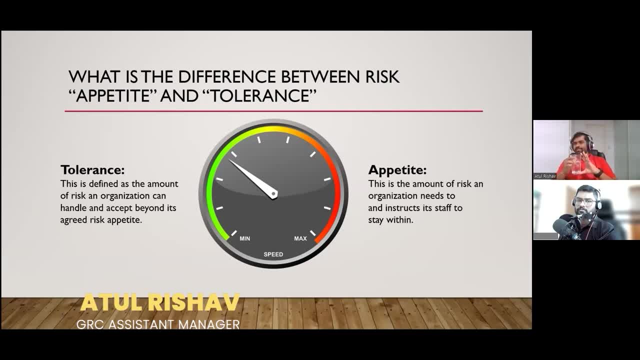 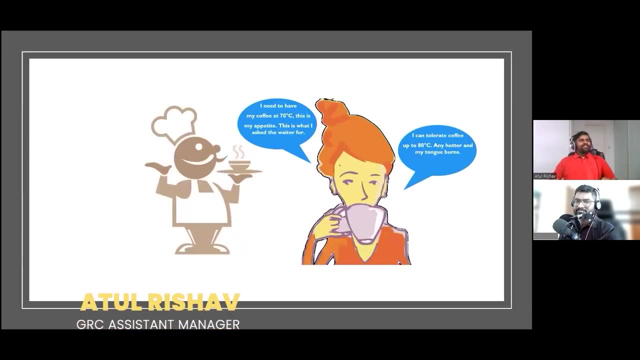 by 10 percent. so this becomes my risk tolerance and I cannot go beyond this right. so I I think I have a good demonstration I was showing, probably before we started to record, so I I think that will make more sense for us to go through, all right. so here it is this: this lady who is sipping her coffee. 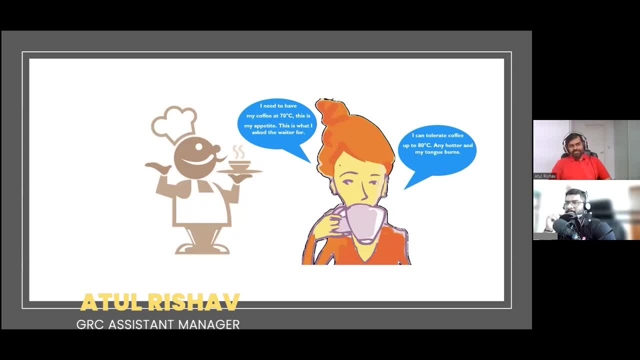 who ordered her coffee and she addresses her, addresses the waiter that you know. uh, she decided beyond 70 degrees and that's that's. that's becomes her risk appetite. this is what she's been in instructed to do and it is what she has instructed to the waiter: that should not go beyond 70 degrees. 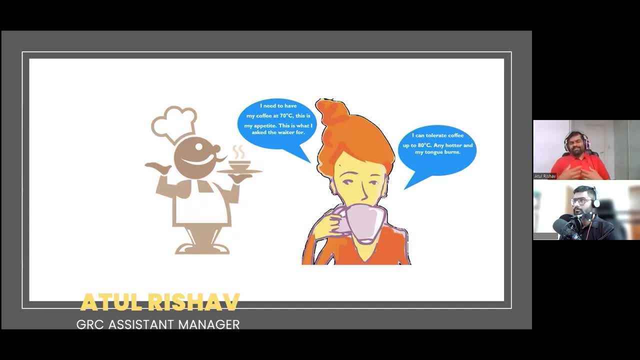 but she knows that life is not perfect, right it, life does not go as planned. so she says that, all right, i can tolerate. i can tolerate by 10 degrees maybe, even if the waiter goes beyond 70, somewhere between 70 to 80, i can tolerate. however, if it gets any hotter, i'm gonna smash that. 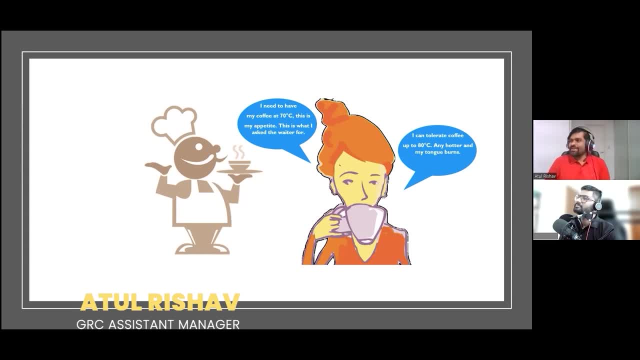 coffee i'm gonna get get. get back my money, i'm not going to going, gonna go back to that coffee shop again, right? so that's exactly. so. that's the. that's the difference, that's the difference between risk appetite and risk. uh, risk tolerance, now in, in, in in cyber security, if you have, if i. 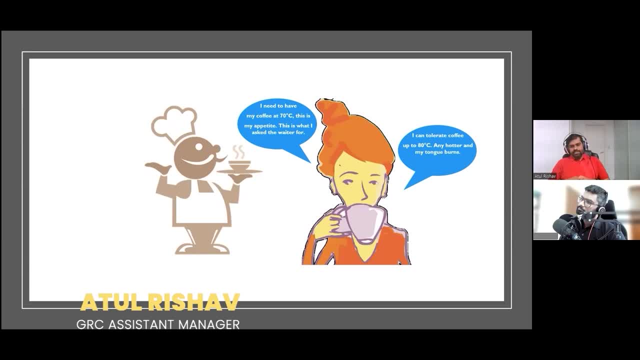 have to speak it, if, if i have to speak it about, uh, from cyber security perspective, say that for me, uh, for all the workstation, sorry for all the servers that i'm looking at. right, my risk appetite is low. i cannot go beyond low. i even cannot afford a medium risk, medium residual risk. 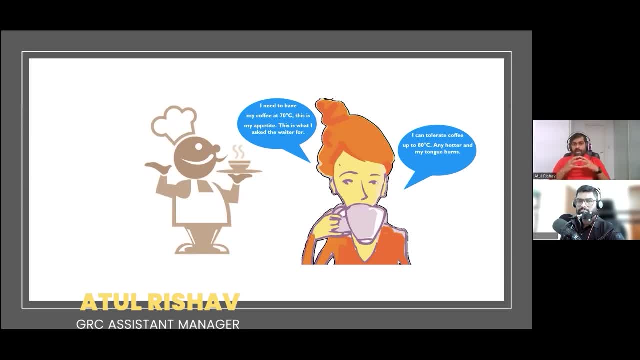 risks to be there. my appetite is low now. i need to make sure that whatever risks that we have identified as an organization should have the residual risk as low. if it is medium, it's best that you look for a new job, maybe right right. so that's, that's the kind of. that's the kind of. 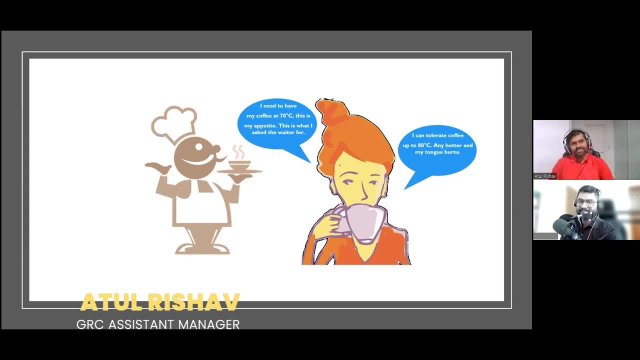 that's, that's how business works, right, so that's the outcome, right, so that's my. that becomes my risk appetite. in this case, in real, in real life scenario, the term risk tolerance i would say i wouldn't say it's non-existence, but at the same time it's understandable. it's understandable that 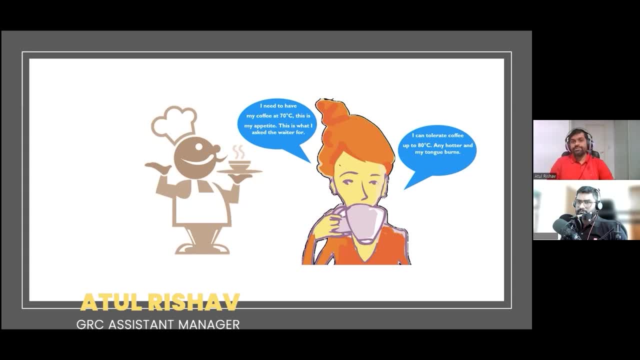 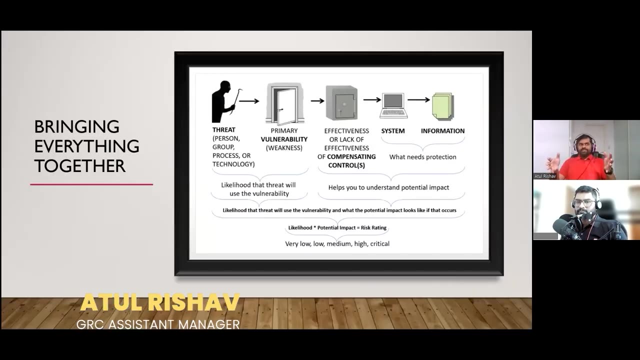 for me, uh, risk appetite is something that i need to adhere to, right? so i cannot go beyond my defined risk appetite. by the way, that's a great insight, right? thank you all, right? so now that we have understood that what's a threat, what's a vulnerability, what's- uh, you know what needs to be protected, what's a likelihood, what? 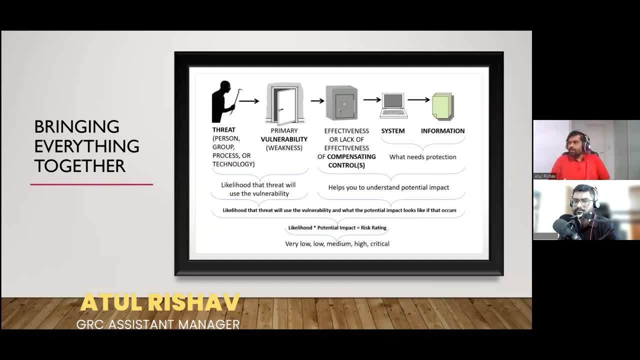 is an impact, let's, let's bring everything together and let's see how it, how it makes sense, right? so, before i take this example, uh, i would also, uh, probably uh, spend a minute on what is a control, right? so it oftentimes people get confused before i mean. 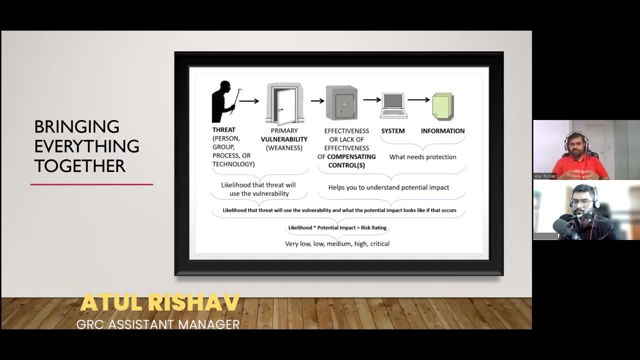 on the definition of control as well. so a control is nothing but a set of instruction, a set of tools, technology, process, people. anything that you have at your disposal, implement to make sure that the risk doesn't occur or at least, if it is accurate, it is below your acceptable level, the risk. 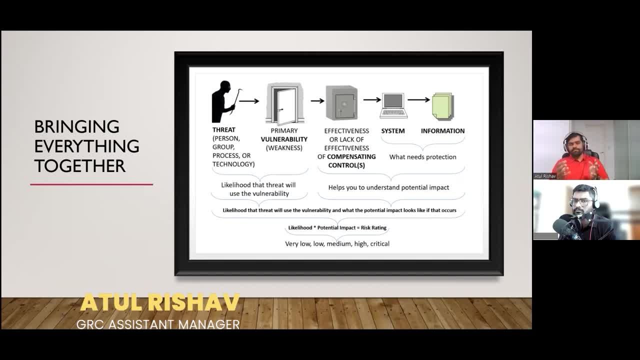 acceptable level that we have spoken about. so that is a control right. a compensating control is something wherein, if you don't have the capability or if you don't have the recommended or ideal control in place at the moment, you have a set of different controls which should act as a substitute, which is not ideal, but that will. that will do the work till. 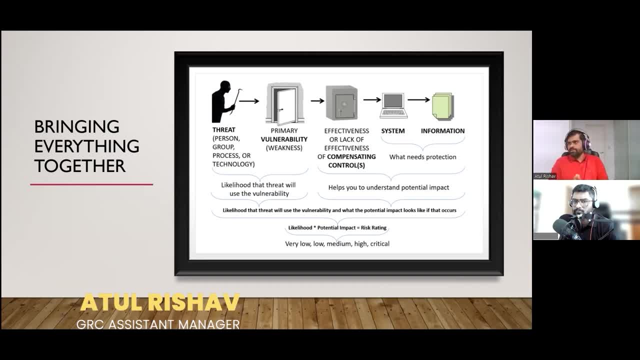 you actually implement the base control or the recommended control, so that's a, that's a compensating control, all right. so let's take this example. it's an, it's an interesting one, so it's a real life example, probably, and then we'll take one, uh, one example from cyber security, and then we move. 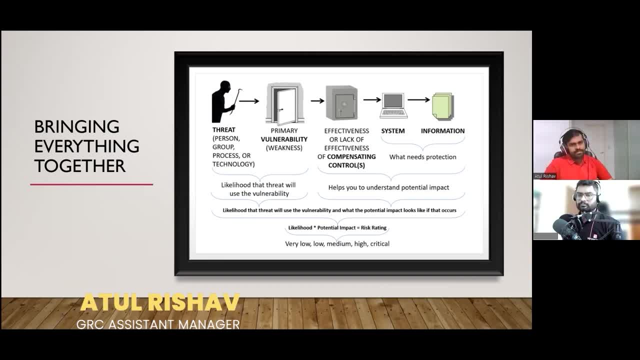 on to the excel sheet that i was sharing with you. all right, so let's pretend. let's pretend that i stay in one of the suburbs in australia, that i do right and i know that the cases of you know, the cases of theft and stealing and whatnot. it's quite prevalent in the suburb that. 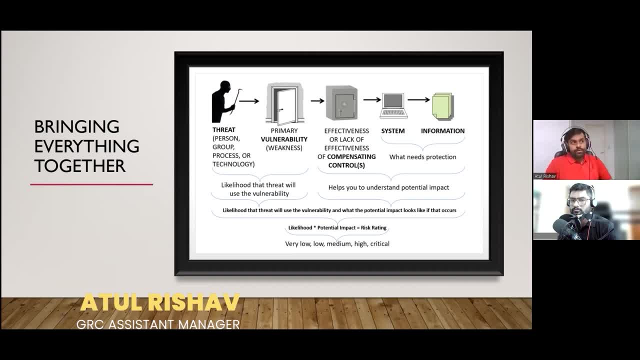 i stay right, even though i know so. in this case, the thief becomes the threat. so a threat could be a person, a group. it can. it can be a process, it can be. it can be a bot as well, right, you know somebody, somebody implementing a bot, somebody writing a bot into python script, and you know. 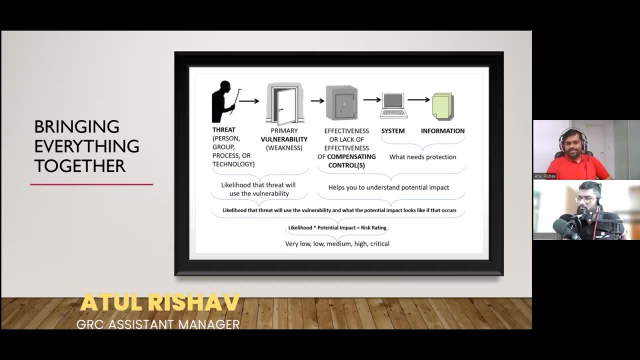 just automating the entire, entire entire stuff for you, right? so in this case, the, the the thief becomes the threat for me. now, to me i. what i should have done is i should have locked my door. ideally, i should have locked my door right, but on one, fine. 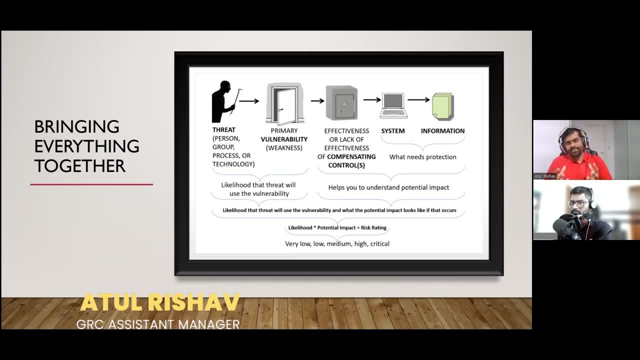 day i lose my mind. i had a glass of beer. i forgot to lock my door. i went off to for shopping and that becomes my vulnerability. that's a vulnerability point for me, right. so for for a threat, or for a for a thief, that becomes a, that becomes an. 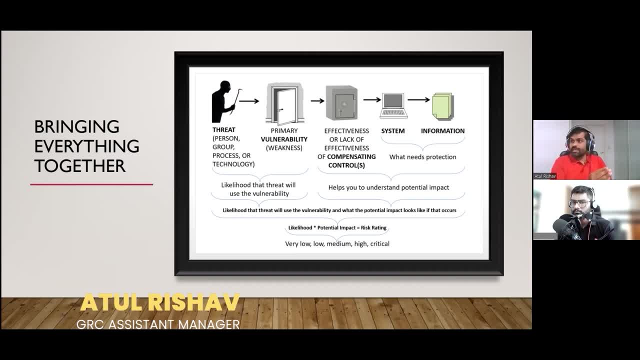 entry point, right that's. that's a primary entry point and that's the known vulnerability. so we know, we know as as probably as human being, we know- that if the house is unlocked, there's a high chance that you know people are going or the thieves are going to wipe off the entire house. 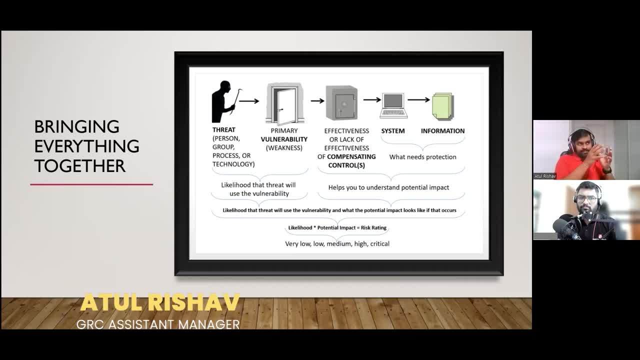 right. so that is. that is one of the weak points and the threat actor, who is quite prevalent in the suburb that i live. he comes to know that i have not locked my door and he was following me for quite some time. right now he enters the house. 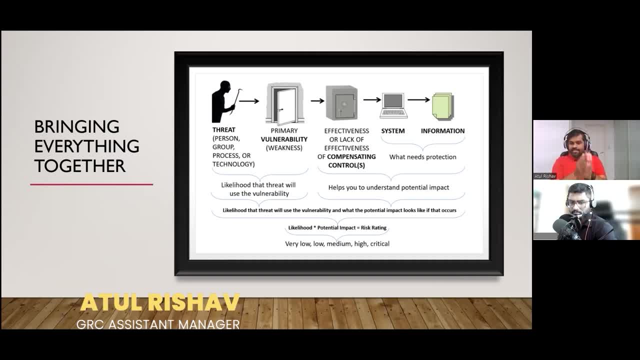 he exploited the vulnerability and he- uh, he exploited the vulnerability, which is a threat, and he actually did that. he entered into the house. now, when he entered into the house, he saw that there's a safe right and he entered into the house and he saw that there's a safe right and he. 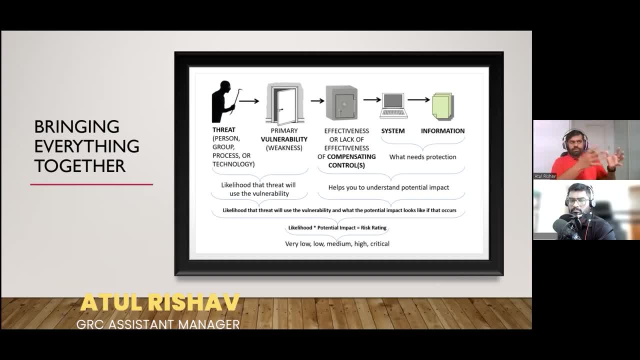 saw that there's a safe right and he entered into the house and he saw that there's a safe right and that safe there's a laptop. i mean not from his perspective, from my perspective. there's a laptop and there's a bunch of document- confidential and restricted documents- from my organization. 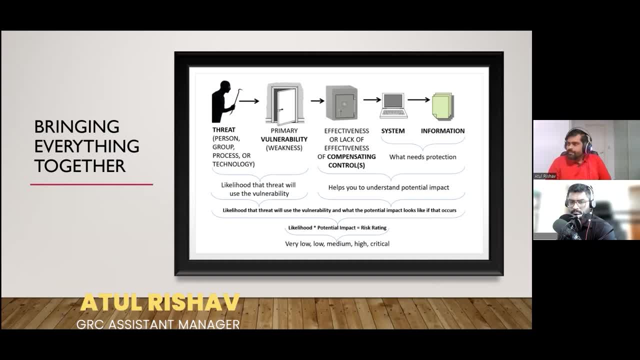 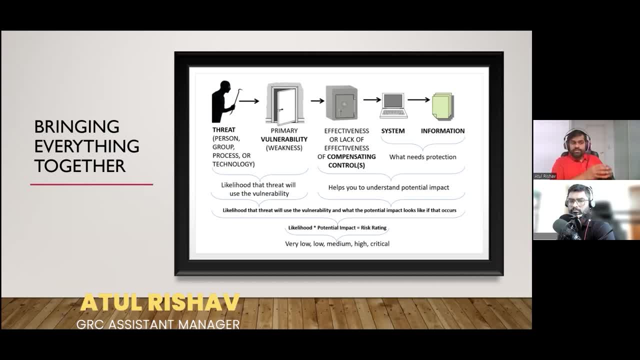 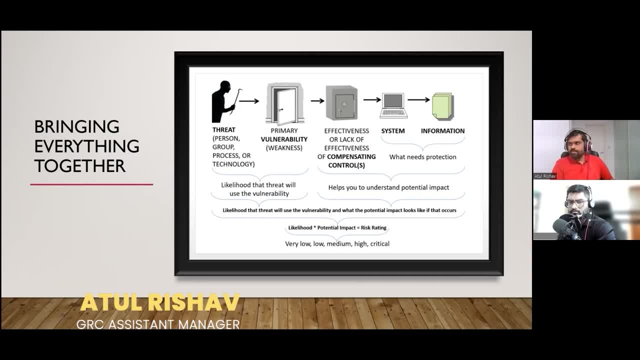 you cannot reveal the confidential or the restricted data, even to your family members. restricted data, even to your family members. restricted data, even to your family members, even to your closed ones, right so, in this case, even to your closed ones, right so, in this case, even to your closed ones. right so in this case, uh, i've got, i've got a laptop with you know. 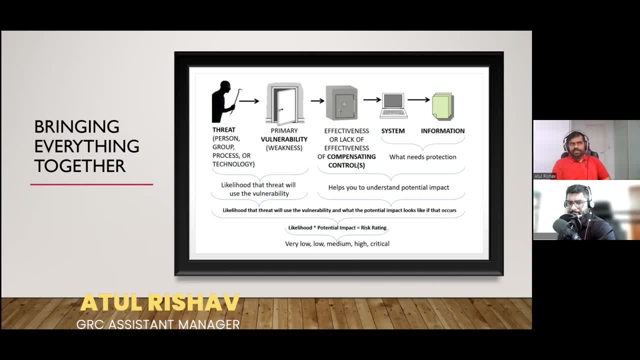 uh, i've got, i've got a laptop with you know. uh, i've got, i've got a laptop with you know, uh, with a lot of information on that, and uh, with a lot of information on that, and uh, with a lot of information on that, and unfortunately there's no bit locker. 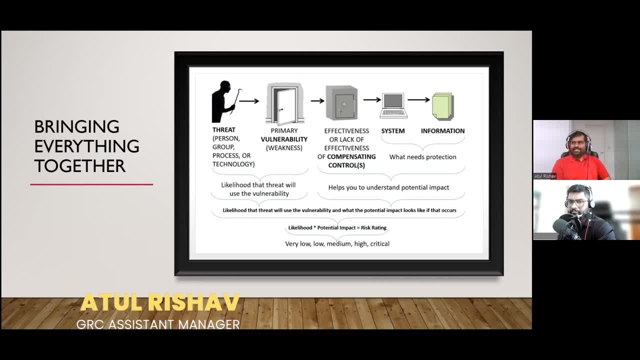 unfortunately there's no bit locker. unfortunately there's no bit locker because the company did not have the, because the company did not have the, because the company did not have the budget for it. right and they put a lot budget for it. right, and they put a lot. 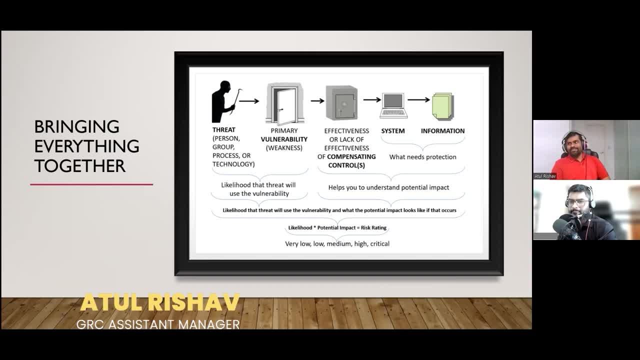 budget for it, right. and they put a lot of trust in me, which is lost now, and uh of trust in me, which is lost now, and uh of trust in me, which is lost now, and uh, i've got bunch of other documents printed. i've got bunch of other documents printed. 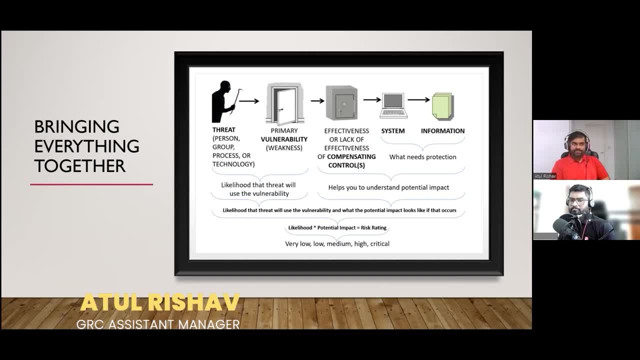 i've got bunch of other documents printed, documents which is quite restricted documents which is quite restricted documents which is quite restricted, which is quite confidential to the firm, which is quite confidential to the firm, which is quite confidential to the firm, and if it is, if it, if it is out. 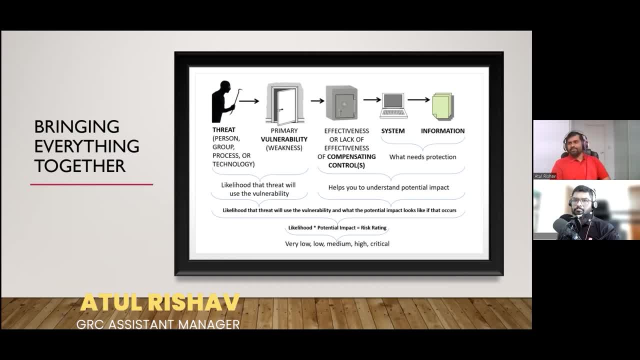 and if it is, if it, if it is out, and if it is, if it, if it is out, uh, the threat actor could easily ask for. uh, the threat actor could easily ask for. uh, the threat actor could easily ask for this. they break it, they get this, they get. 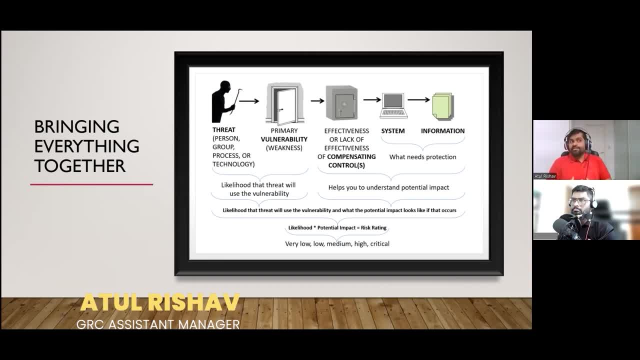 this, they break it, they get this, they get this, they break it, they get this, they get hands on to the system and the hands on to the system and the hands on to the system and the information, information, information. what is it? this is the impact. that's. 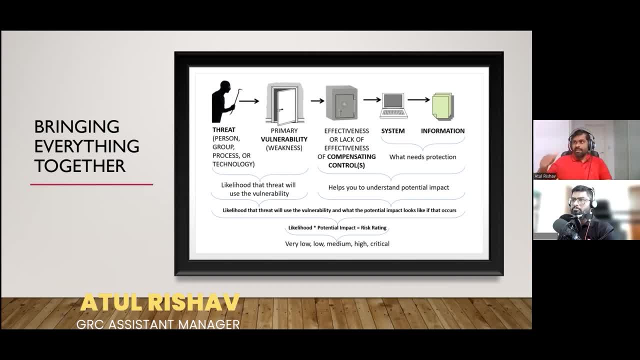 what is it? this is the impact. that's what is it. this is the impact that's going to be on the organization. so a going to be on the organization. so a going to be on the organization. so a threat actor exploiting the vulnerability. threat actor exploiting the vulnerability. 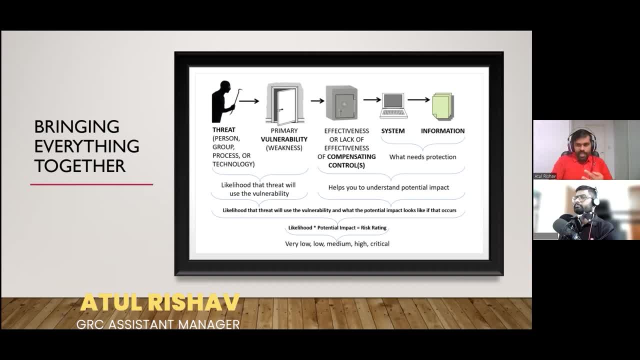 threat actor exploiting the vulnerability: uh, you know and uh uh, you know and uh uh, you know and uh, having having this incident. you know having having this incident. you know having having this incident. you know the incident definition when we uh we. the incident definition when we uh we. 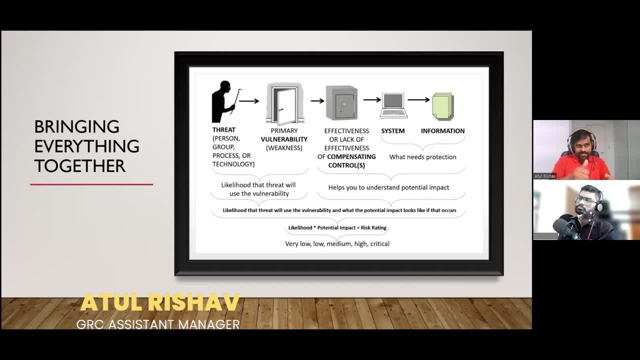 the incident definition when we uh we spoke about earlier. i guess so uh now spoke about earlier. i guess so uh now spoke about earlier. i guess so, uh, now there's this incident wherein the there's this incident, wherein the there's this incident wherein the threat actor actually has hands-on to. 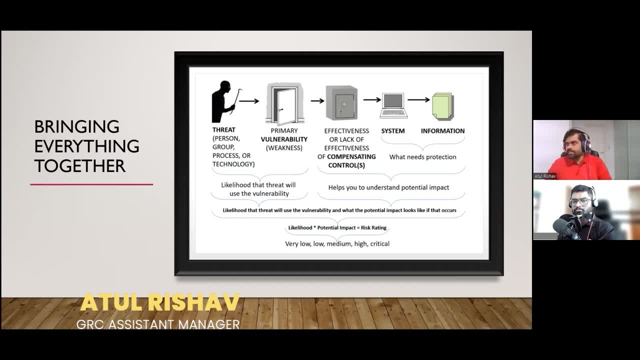 threat actor actually has hands-on to threat actor actually has hands-on to the system and the information that the system and the information that the system and the information that becomes a potential impact becomes a potential impact, becomes a potential impact on the organization and on you: on the organization and on you. 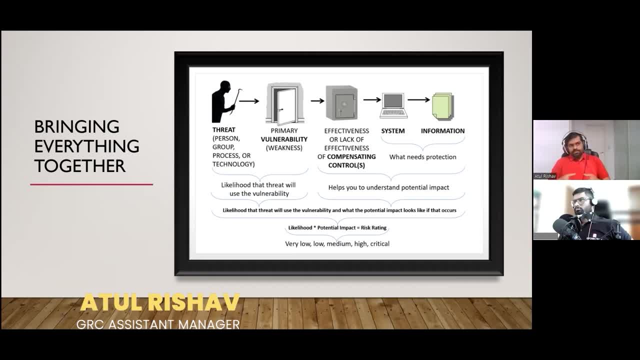 on the organization and on you personally as well. right, so in general, personally as well. right, so in general, personally as well. right, so in general cases, or in general sense the risk cases, or in general sense the risk cases, or in general sense, the risk rating, is calculated as a potential. 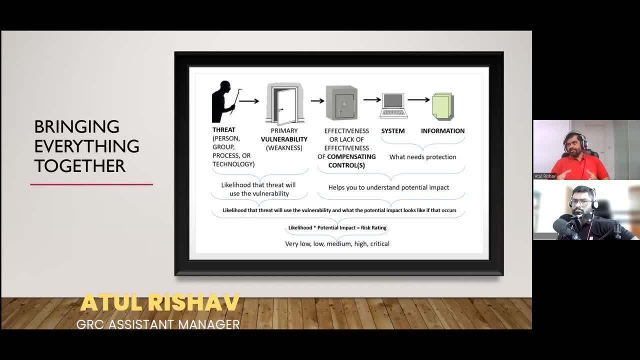 rating is calculated as a potential rating is calculated as a potential impact times likelihood. so this is the impact times likelihood. so this is the impact times likelihood. so this is the general understanding. it could differ general understanding. it could differ general understanding. it could differ from company to company depending on the 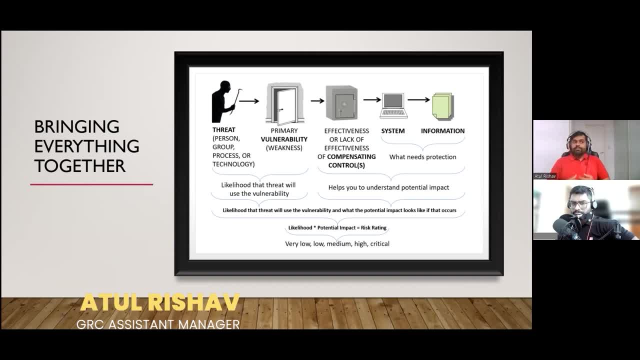 from company to company, depending on the from company to company, depending on the size, depending on the complexity of the size, depending on the complexity of the size, depending on the complexity of the organization, they might also consider organization. they might also consider organization. they might also consider the asset value into the picture, if you. 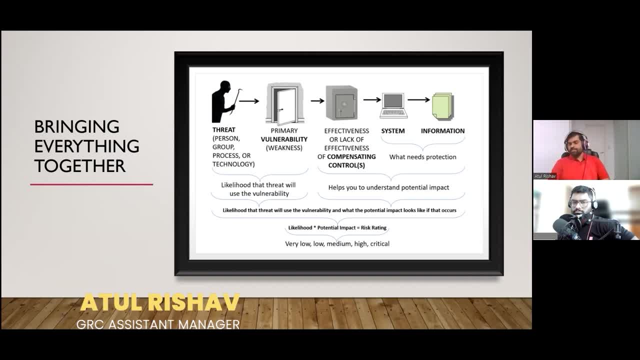 the asset value into the picture, if you the asset value into the picture, if you are going, if they are going for uh are going. if they are going for uh are going. if they are going for uh. quantitative uh assessment of the risk. quantitative uh assessment of the risk. 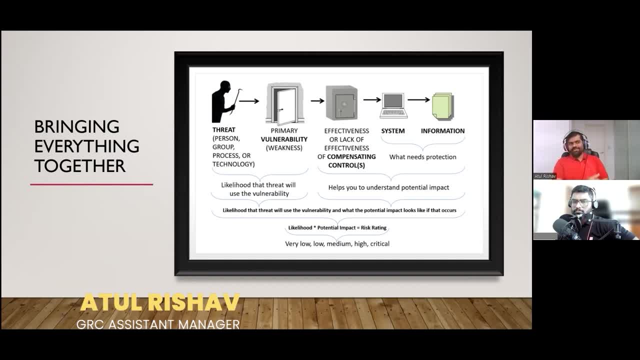 quantitative uh assessment of the risk. so this is one of the real life example. so this is one of the real life example. so this is one of the real life example- or probably analogy, or probably analogy, or probably analogy- that i tried to connect with the. that i tried to connect with the. 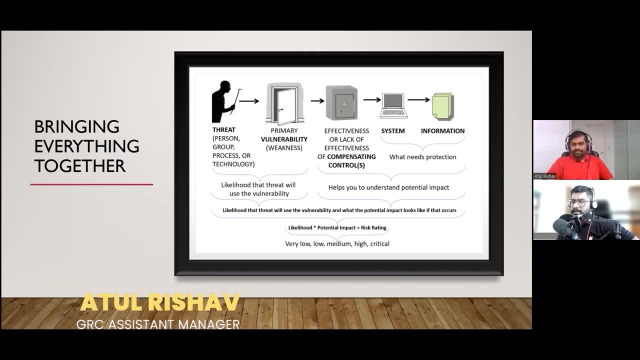 that i tried to connect with the definitions that we discussed earlier, definitions that we discussed earlier, definitions that we discussed earlier. that is that it's really great and uh it, that is that it's really great and uh it, that is that it's really great and uh, it is good to see that. you know you're. is good to see that you know you're is good to see that you know you're using a real life analogy, because, if using a real life analogy, because, if using a real life analogy, because if you're going with the technical things, you're going with the technical things. 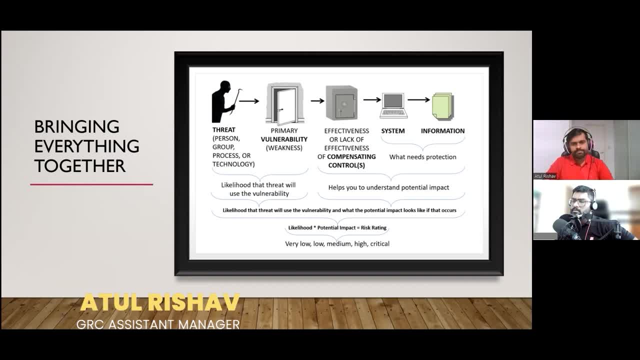 you're going with the technical things and all that- not everyone really. and all that, not everyone really. and all that, not everyone really. absolutely, yeah, that's that's okay. absolutely yeah, that's that's okay. absolutely yeah, that's that's okay. that's a. that's the best thing. 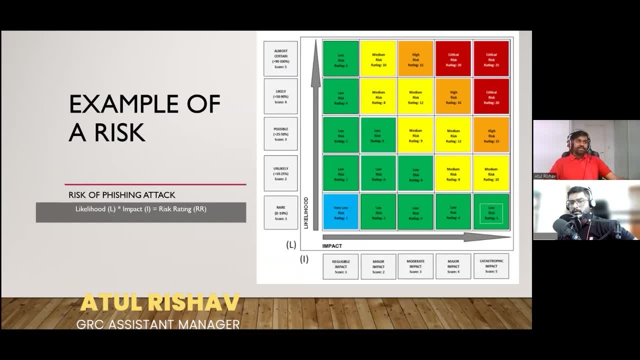 that's a, that's the best thing. that's a that's the best thing. yeah, absolutely, yeah, absolutely, yeah, absolutely so, having said that now, so, having said that now, so having said that now, no, let's take a, let's, let's take an. no, let's take a, let's, let's take an. 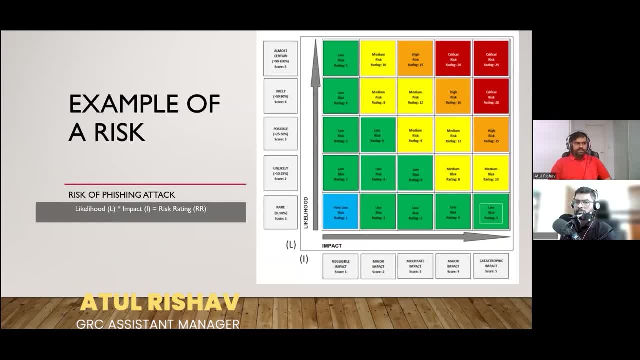 no, let's take a. let's let's take an example from cyber security industry, example from cyber security industry, example from cyber security industry. right so phishing attack. right so phishing attack. right so phishing attack. there's always a risk of phishing attack. there's always a risk of phishing attack. there's always a risk of phishing attack. right. say that your email servers are right. say that your email servers are right. say that your email servers are not appropriately configured. if you not appropriately configured, if you not appropriately configured, if you don't have, if you don't have a proper. 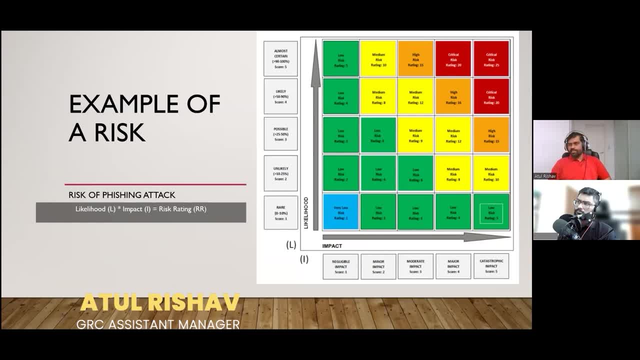 don't have. if you don't have a proper, don't have. if you don't have a proper dlp, sorry. a proper email filtering or dlp: sorry. a proper email filtering or dlp. sorry. a proper email filtering or url filtering mechanism. you know url filtering mechanism, you know. 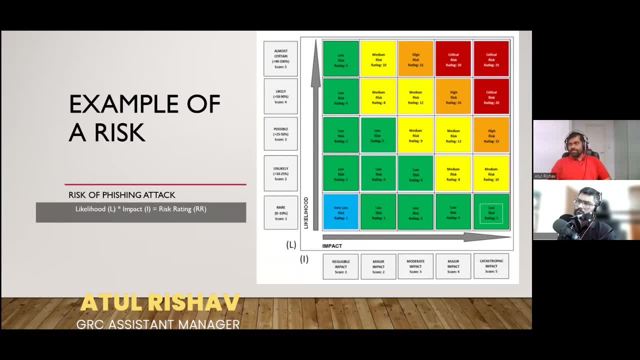 url filtering mechanism, you know, implemented in the company. there's implemented in the company. there's implemented in the company. there's always a risk that you would be always a risk, that you would be always a risk that you would be receiving a phishing email. receiving a phishing email. 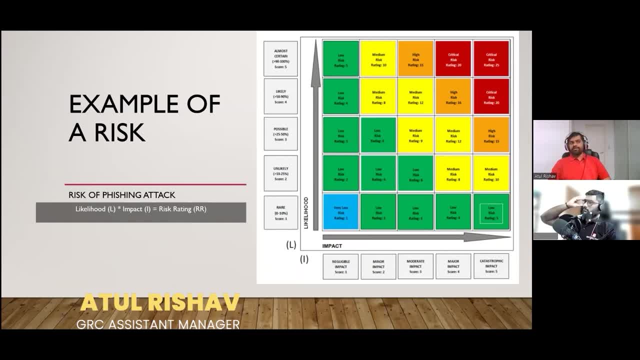 receiving a phishing email to your employees and if one of the to your employees and if one of the to your employees and if one of the employees fell for it, that's all it takes. employees fell for it, that's all it takes. employees fell for it, that's all it takes. right could be data breach could be. 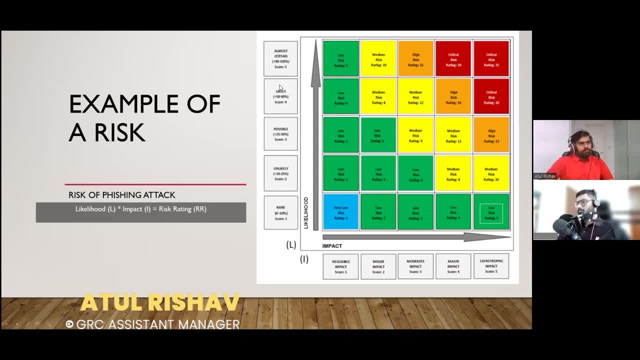 right could be data breach could be right could be data breach. could be malware injection and whatnot. right. so malware injection and whatnot? right? so malware injection and whatnot. right. so let's, let's understand that. what would? let's, let's understand that. what would? 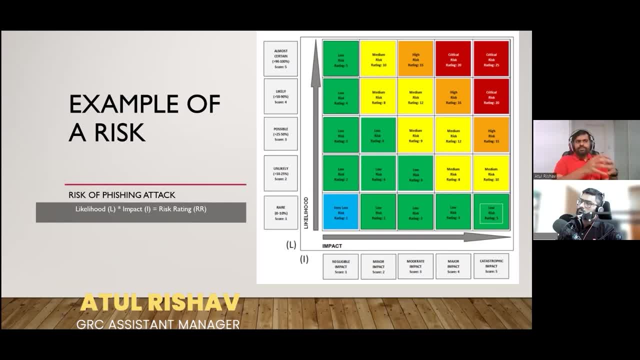 let's, let's understand that. what would be the risk rating here, right? so be the risk rating here, right so be the risk rating here, right so, in the worst case scenario, if the in the worst case scenario, if the in the worst case scenario, if the company does not have any control of the 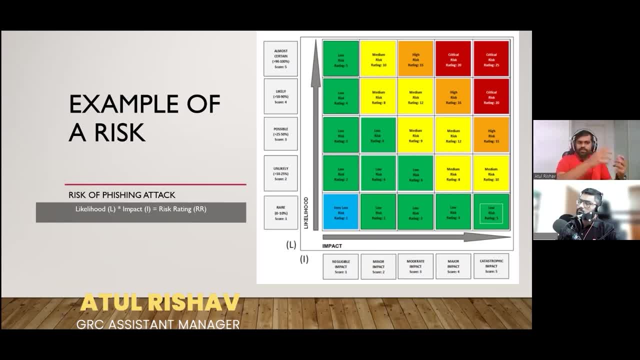 company does not have any control of the company does not have any control of the of the tools and technologies that they, of the tools and technologies that they, of the tools and technologies that they have implemented and they have not have implemented and they have not have implemented and they have not configured it properly. they have not 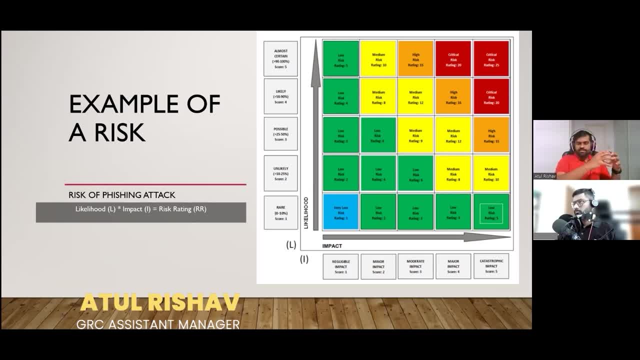 configured it properly. they have not configured it properly, they have not implemented it properly. so mistake, let's implemented it properly. so mistake, let's implemented it properly. so mistake, let's understand from that perspective right, understand from that perspective right, understand from that perspective right. in that case, the likelihood of getting 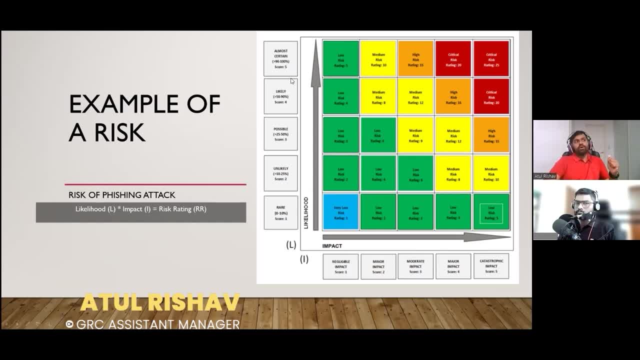 in that case, the likelihood of getting, in that case, the likelihood of getting, a fishing email to your employees, a fishing email to your employees, a fishing email to your employees, becomes almost certain, which is a five becomes almost certain, which is a five becomes almost certain, which is a five. i would probably have a pointer here. 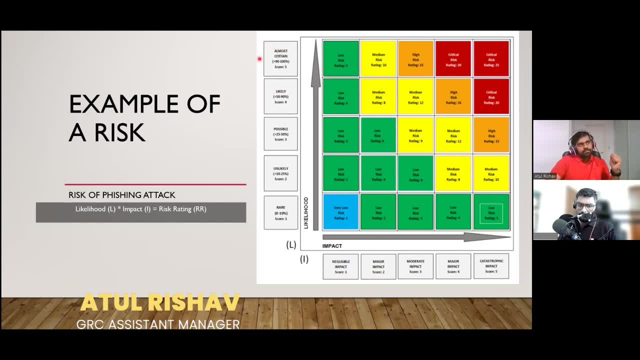 i would probably have a pointer here, i would probably have a pointer here, so so, so i hope this is fine, all right. so i hope this is fine, all right. so i hope this is fine, all right. so this, this is our likelihood. this, this is our likelihood. 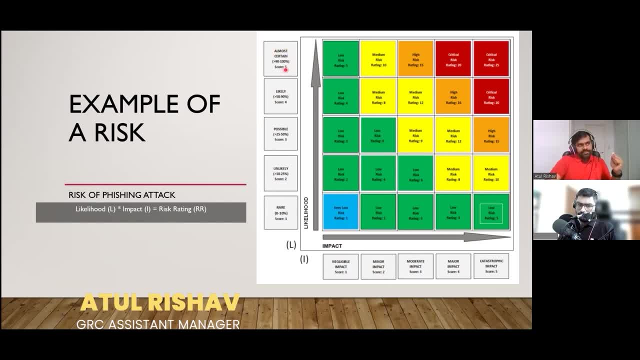 this, this is our likelihood. right so, right so, right so. in in a in a scenario or in a case in in a in a scenario or in a case in in a in a scenario or in a case wherein you don't have anything you, wherein you don't have anything, you. 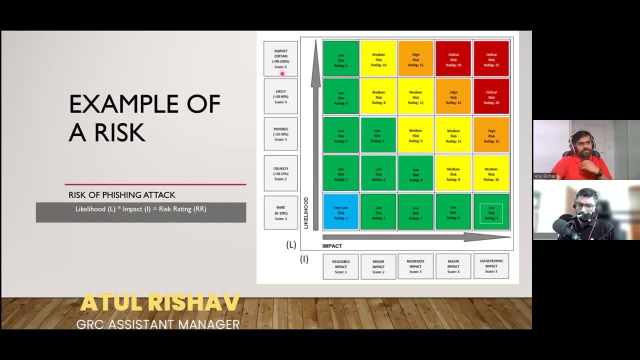 wherein you don't have anything. you don't. i mean i mean you have not don't. i mean i mean you have not don't. i mean i mean you have not configured it properly. you don't have configured it properly. you don't have configured it properly, you don't have anything right. so in that case, the 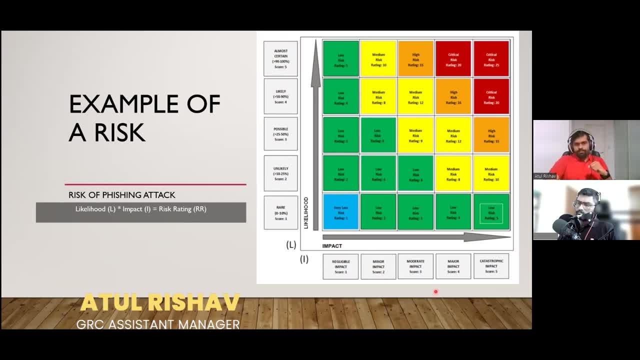 anything right. so in that case, the anything right, so in that case, the likelihood is quite high. likelihood is quite high. likelihood is quite high, however, however. however, the impact that we are looking at, might the impact that we are looking at, might the impact that we are looking at might be full. 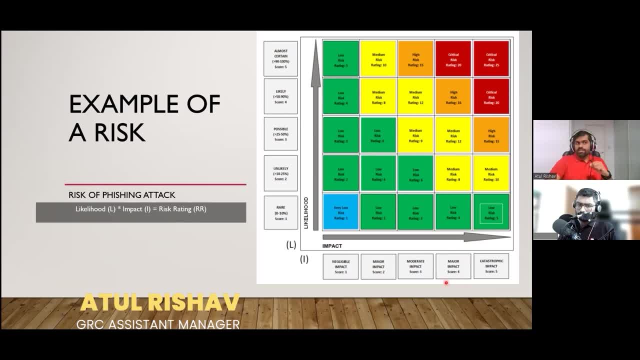 be full. be full. i wouldn't give a catastrophic. because i wouldn't give a catastrophic, because i wouldn't give a catastrophic, because it will always depend that who is. it will always depend that who is. it will always depend that who is receiving the phishing email, if it is. 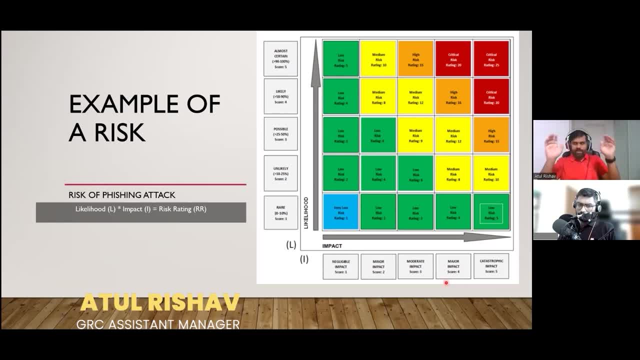 receiving the phishing email. if it is receiving the phishing email, if it is your admin team, your admin team, your admin team. i don't care about it. right, i will. i don't care about it. right, i will. i don't care about it. right, i will probably give the data myself. 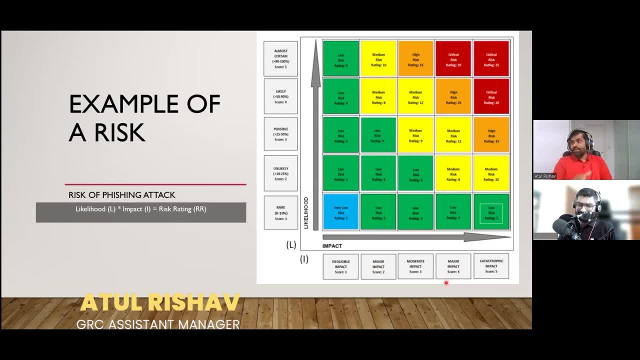 probably give the data myself, probably give the data myself to the actors, to the threat actors. right to the actors. to the threat actors. right to the actors. to the threat actors, right. but what if one of your admin one of? but what if one of your admin one of? 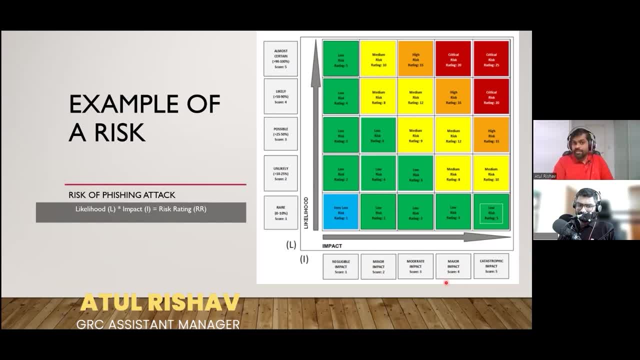 but what if one of your admin, one of your id team members? what if one of your your id team members? what if one of your your id team members, what if one of your board members who is holding quite board members, who is holding quite board members, who is holding quite critical and sensitive information? 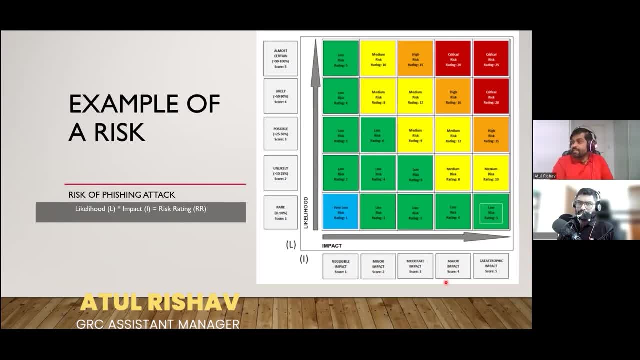 critical and sensitive information. critical and sensitive information: receives the phishing link. and receives the phishing link. and receives the phishing link. and and they actually click on it, right so, and they actually click on it, right so, and they actually click on it, right so, keeping those subjective scenarios and 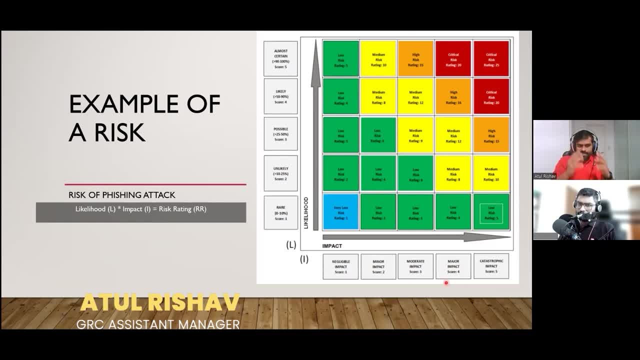 keeping those subjective scenarios and keeping those subjective scenarios and keeping those uh subjective, keeping those uh subjective, keeping those uh subjective aspects in mind. i would probably rate it aspects in mind. i would probably rate it aspects in mind. i would probably rate it as a four, as a four. 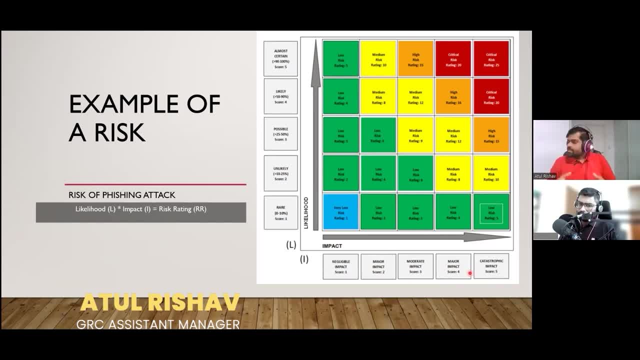 as a four now, now, now, going back to my previous estate, right, going back to my previous estate, right, going back to my previous estate, right, every company would have, every company would have, every company would have, uh, their own approach, uh, their own approach, uh, their own approach for conducting risk assessment. they. 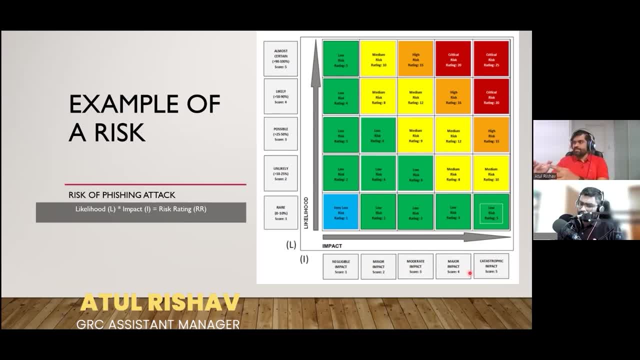 for conducting risk assessment. they for conducting risk assessment. they could go for quantitative assessment, could go for quantitative assessment, could go for quantitative assessment. they could also go for qualitative. they could also go for qualitative. they could also go for qualitative assessments. so the the scenario that we assessments. so the the scenario that we. 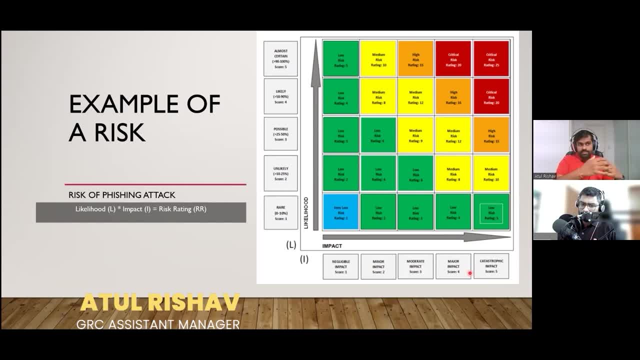 assessments. so the the scenario that we are discussing here is a qualitative. are discussing here is a qualitative. are discussing here is a qualitative approach. it's based on the experience approach. it's based on the experience approach. it's based on the experience. it's based on the known vulnerabilities. 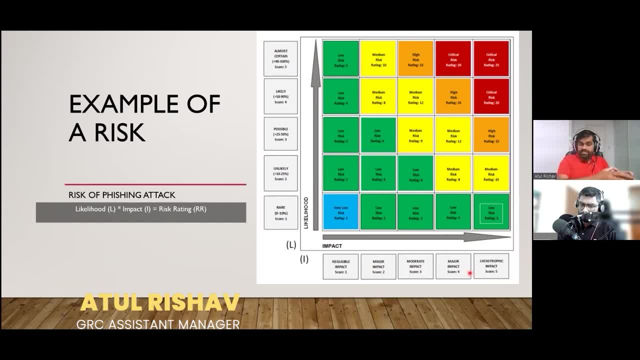 it's based on the known vulnerabilities. it's based on the known vulnerabilities. it's based on the known threats to the. it's based on the known threats to the. it's based on the known threats to the industry, or industry or industry or uh, to the similar size of the company. 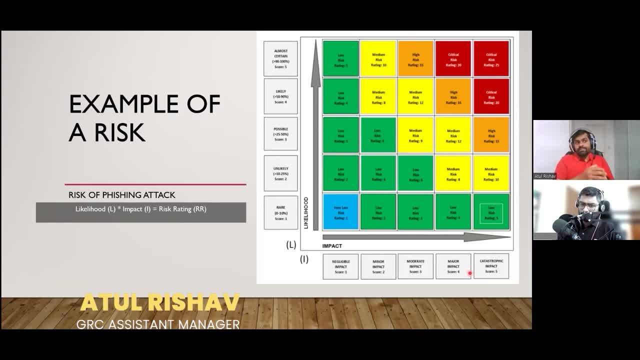 uh to the similar size of the company. uh to the similar size of the company. would go for quantitative risk assessment. would go for quantitative risk assessment. would go for quantitative risk assessment because it's it's quite time consuming, because it's it's quite time consuming because it's it's quite time consuming, it's. 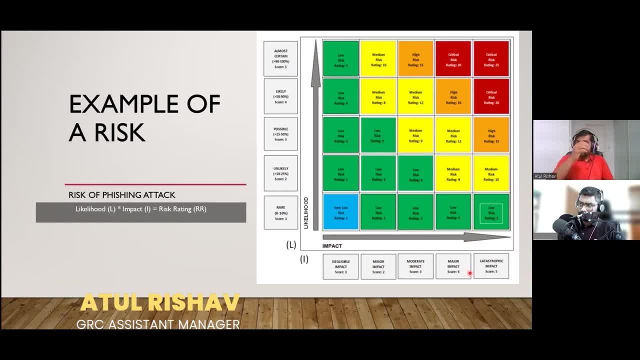 it's it's time consuming. it's it's time consuming. it's. it's really it's it's time consuming. it's. it's really it's it's time consuming it's. it's really complicated. you need really good people complicated. you need really good people. 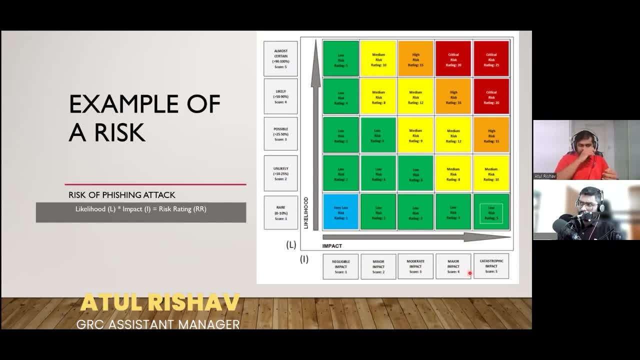 complicated. you need really good people to you know work on it and invest time to you know work on it and invest time to you know work on it and invest time on it right. so that usually happens in on it right. so that usually happens in on it right. so that usually happens in some larger companies that we are in. 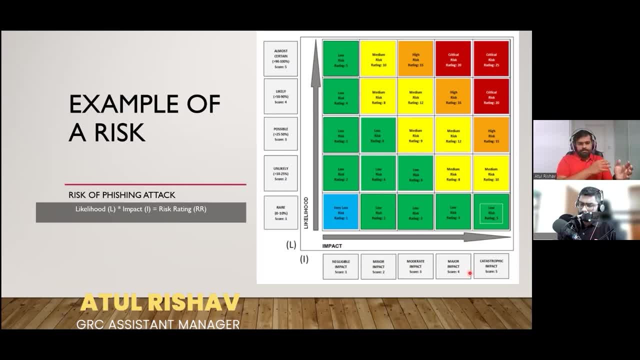 some larger companies that we are in, some larger companies that we are in wherein they actually need to go for, wherein they actually need to go for, wherein they actually need to go for they have like, they have like, they have like, uh, tens of thousands of workstations and 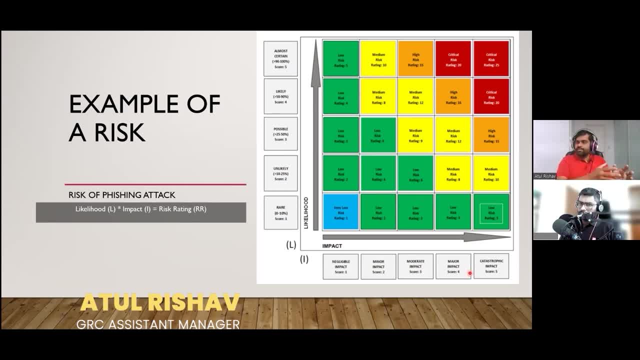 uh, tens of thousands of workstations and uh, tens of thousands of workstations and servers and what nots within the servers and what nots within the servers and what nots within the organization organization, and they organization, organization and they organization organization. and they actually need to look at that. what is? 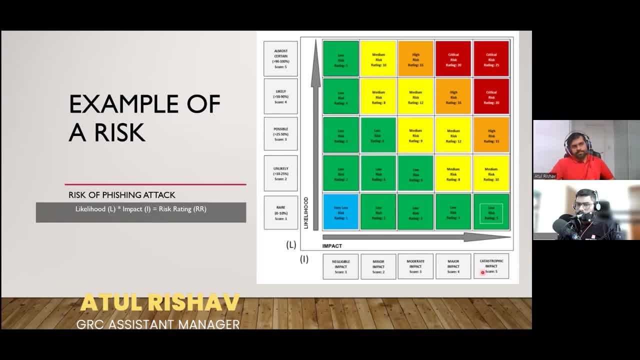 actually need to look at that. what is actually need to look at that. what is the monetary loss that we are looking at, the monetary loss that we are looking at, the monetary loss that we are looking at, now coming back to or circling back to, now coming back to or circling back to. 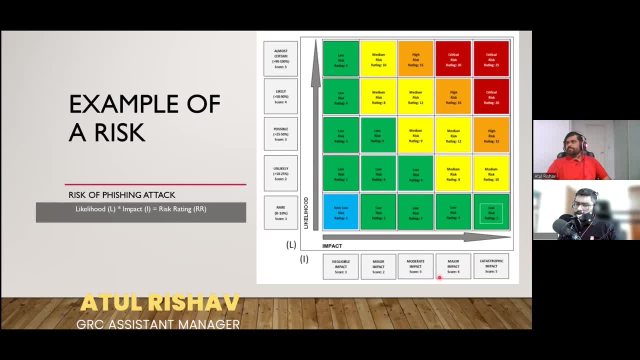 now coming back to, or circling back to, the example that we were discussing, the example that we were discussing, the example that we were discussing. sorry to interrupt here. actually, yeah, sorry to interrupt here, actually, yeah, sorry to interrupt here. actually, yeah, sure, sure. when it comes to the impact, 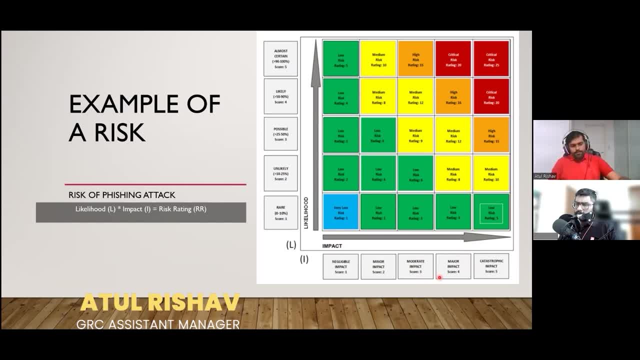 sure, sure when it comes to the impact, sure, sure when it comes to the impact parameter and all that. i believe that is parameter and all that i believe that is parameter and all that i believe that is varies from uh process to process. varies from uh process to process. 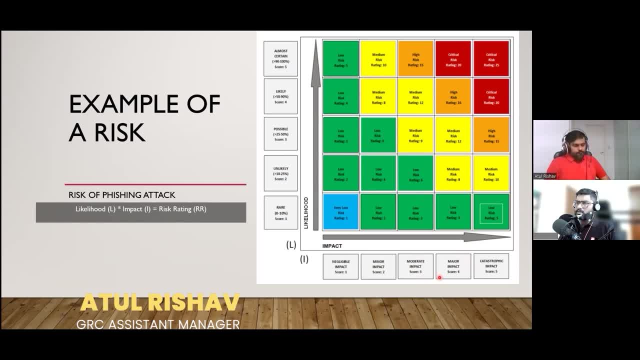 varies from uh process to process. organization might be in that company, organization might be in that company, organization might be in that company. as i said, catastrophic is there but in. as i said, catastrophic is there but in. as i said, catastrophic is there but in other, other other we might have a different perspective. 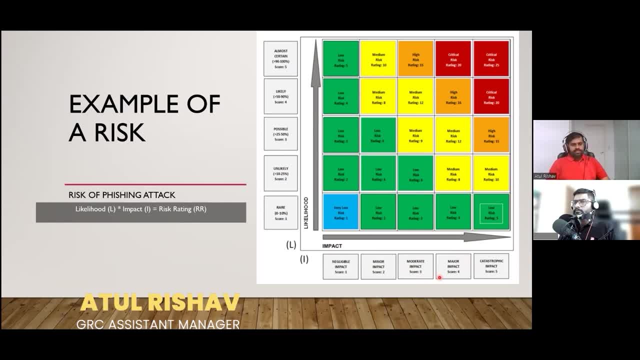 we might have a different perspective. we might have a different perspective. right, exactly, absolutely, you're right. right, exactly, absolutely, you're right, right, exactly, absolutely you're right. so so say that. if, if, if i'm a bpo, so so say that. if, if, if i'm a bpo, 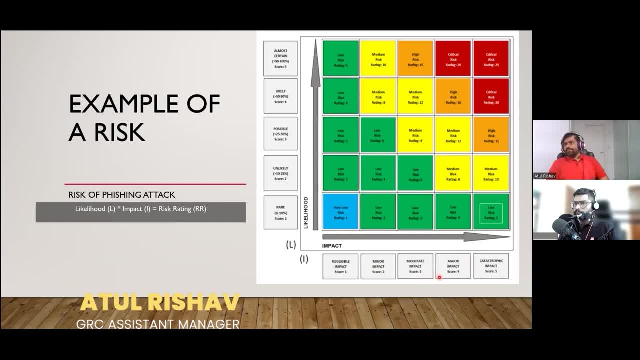 so so say that if, if i'm a bpo right and uh, i don't hold any data for right and uh, i don't hold any data for right and uh, i don't hold any data for that matter, i only do that matter, i only do. 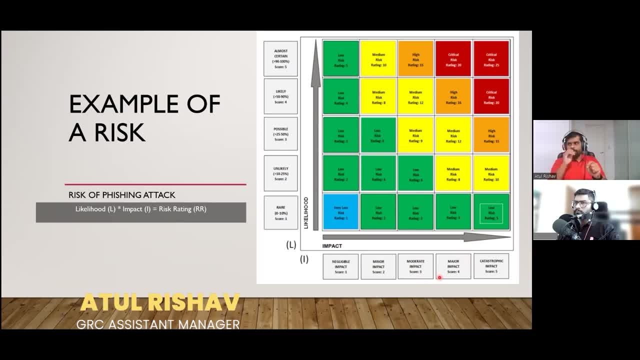 that matter, i only do processing right payroll processing and processing right payroll processing and processing right payroll processing and whatnot, and and that's all i do. i mean whatnot, and, and that's all i do. i mean whatnot, and and that's all i do. i mean, when i say payroll processing, i mean the. 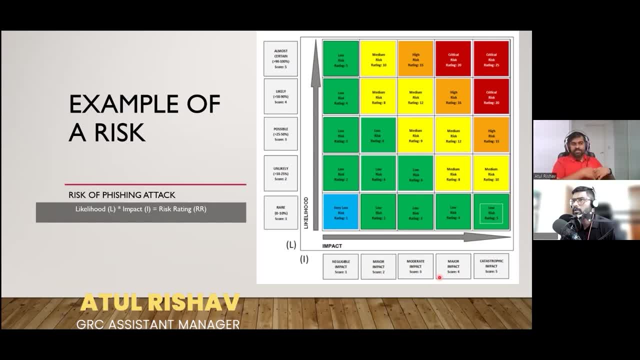 when i say payroll processing, i mean the. when i say payroll processing, i mean the: the paperwork, not the actual payroll. the paperwork, not the actual payroll. the paperwork, not the actual payroll. processing work. right so as a bpo if i'm processing work. right so as a bpo if i'm. 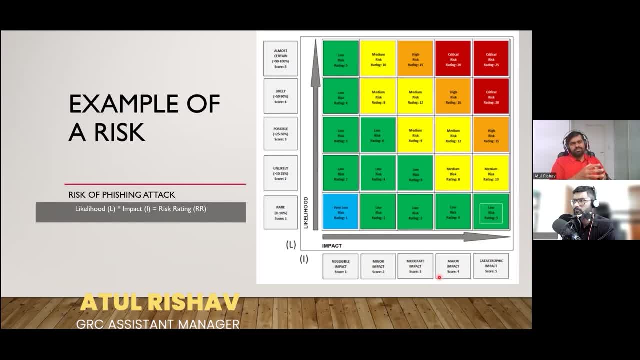 processing work right. so, as a bpo, if i'm a back office, a back office, a back office for me. phishing attack is is not for me. phishing attack is is not for me. phishing attack is is not something that i'd probably look, something that i'd probably look. 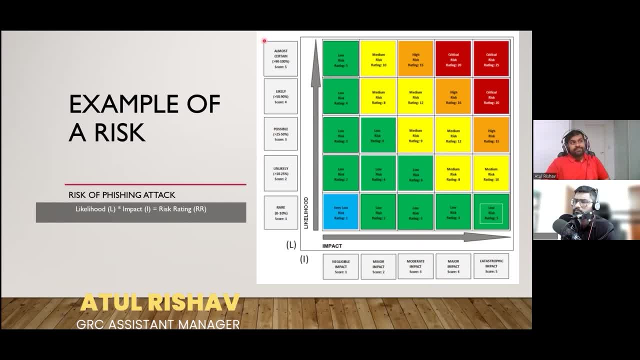 something that i'd probably look, look for right in this in this case. look for right in this in this case. look for right in this in this case. it, it will still be almost certain, but it, it will still be almost certain. but it, it will still be almost certain. but the impact that we are speaking about 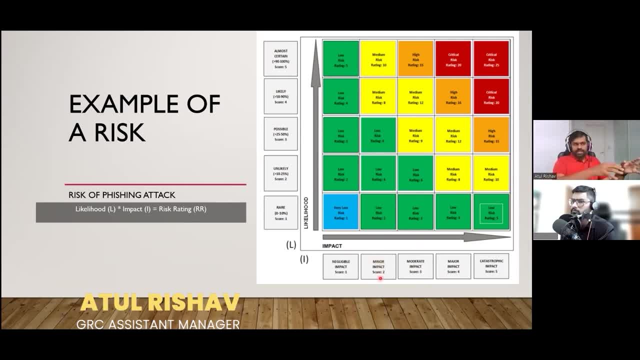 the impact that we are speaking about. the impact that we are speaking about would be minor for me, understood. so, yes, would be minor for me understood. so yes, would be minor for me understood. so, yes, you're right. so in the, the, the idea of you're right. so in the, the, the idea of. 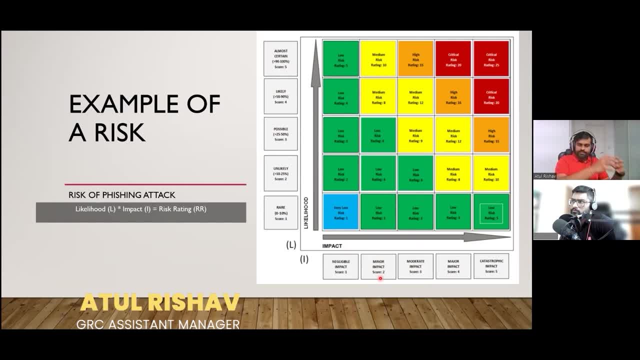 you're right. so in the the, the idea of the idea of risk management or the idea the idea of risk management or the idea, the idea of risk management or the idea of the risk assessment differs from of the risk assessment, differs from of the risk assessment differs from company to company, differs. 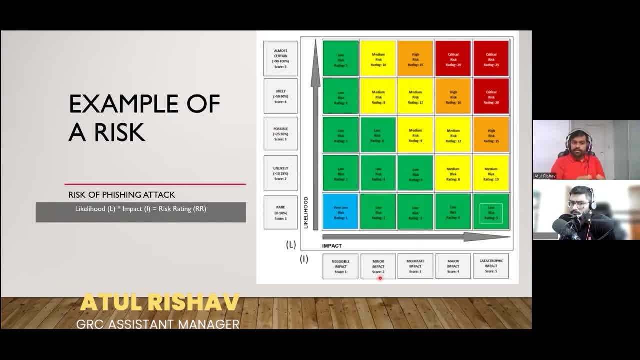 company to company differs. company to company differs from the company. who are actually you from the company? who are actually you from the company? who are actually, you know, working or operating within the know, working or operating within the know, working or operating within the same industry? it depends on the 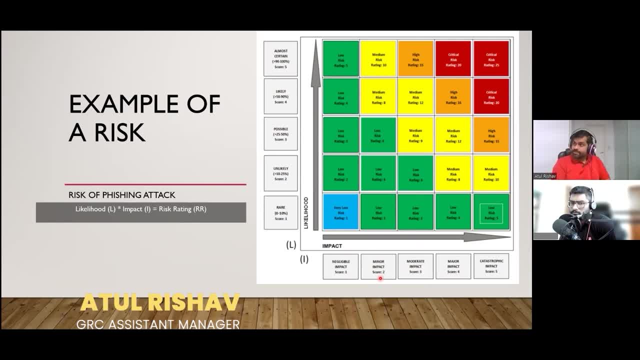 same industry. it depends on the same industry. it depends on the complexity of your writing moment. it complexity of your writing moment. it complexity of your writing moment. it depends on the kind of data that you depends on. the kind of data that you depends on, the kind of data that you hold. you might not hold any data, even. 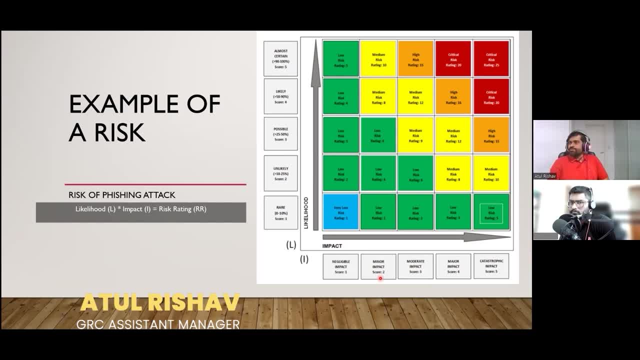 hold, you might not hold any data. even hold, you might not hold any data. even right, you might as well. you would be a right, you might as well, you would be a right. you might as well, you would be a mediator to two firms, and you're not. 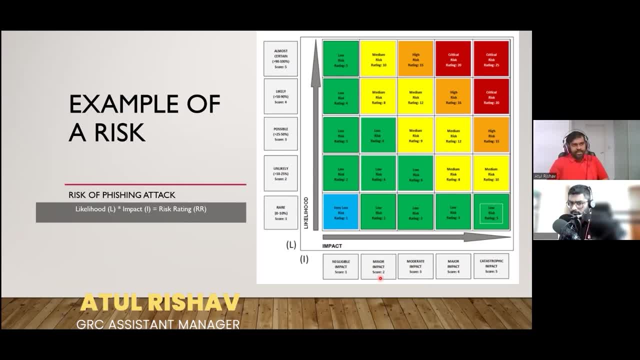 mediator to two firms and you're not mediator to two firms and you're not holding any data. you're just, you're just holding any data. you're just, you're just holding any data. you're just, you're just a mediator to them. right in every case. 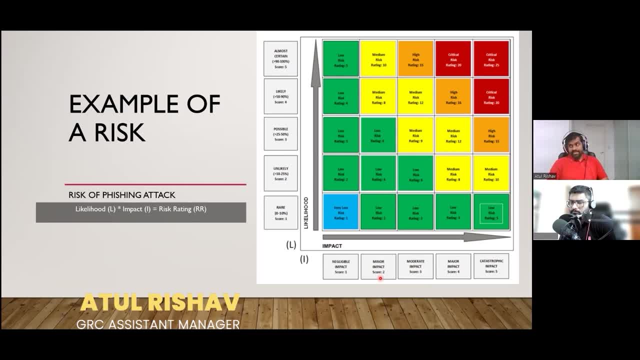 a mediator to them right in every case, a mediator to them right in every case, the impact would differ, however, having the impact would differ. however, having the impact would differ. however, having said that said, that said that the likelihood will still be high. it's, the likelihood will still be high. it's. 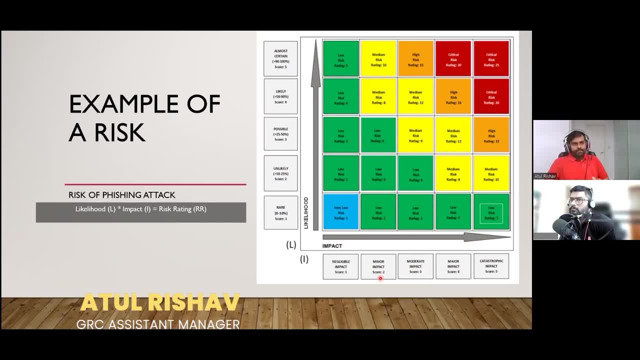 the likelihood will still be high. it's just that the impact would be low. in just that the impact would be low, in just that the impact would be low in every case, every case, every case, right so, right, so, right so uh in in a case, in a case wherein uh. 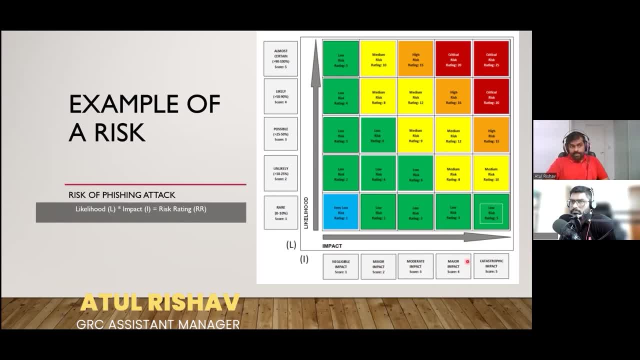 uh. in a case wherein, uh, uh, in a case wherein uh, uh, sensitive industry for me, the impact- uh, sensitive industry for me, the impact- uh, sensitive industry for me, the impact would be major, would be major, would be major. now, mapping it to. so this is called a. 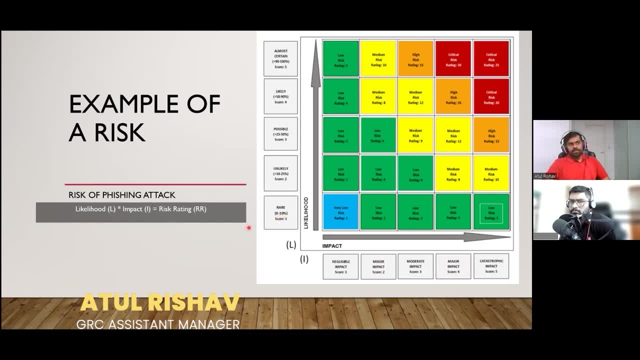 now mapping it to, so this is called a now mapping it to, so this is called a five by five matrix, right? so we have we five by five matrix right, so we have we five by five matrix right, so we have. we have got uh likelihood rated from one to. 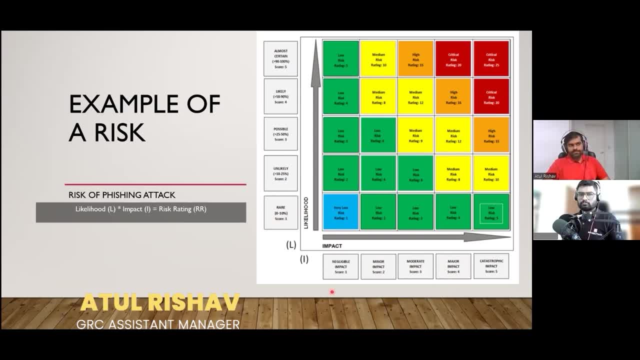 have got uh likelihood rated from one to have got uh likelihood rated from one to five, one being the lowest and five being five, one being the lowest and five being five, one being the lowest and five being the highest- the highest, the highest. likewise for impact, one being the lowest. 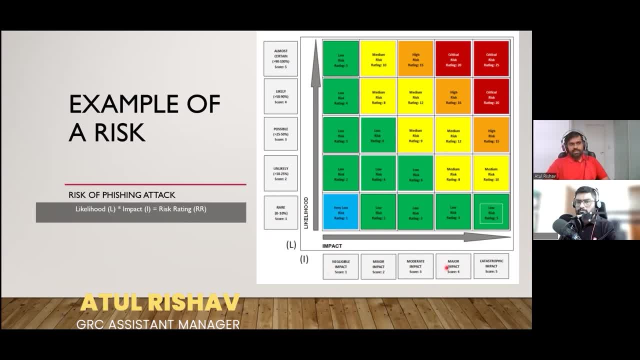 likewise for impact, one being the lowest. likewise for impact, one being the lowest and five being the highest. so this is a, and five being the lowest and five being the highest. so this is a, and five being the lowest and five being the highest. so this is a five by five matrix. so i would, i would. 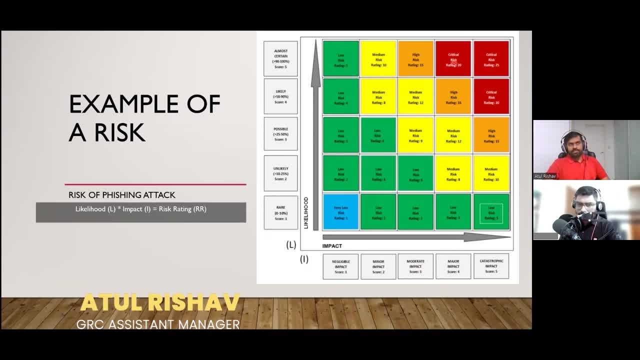 five by five matrix, so i would, i would: five by five matrix, so i would, i would just point that, which matrix does it just point that? which matrix does it just point that? which matrix does it belong? i mean, which quadrant does it belong? i mean, which quadrant does it? 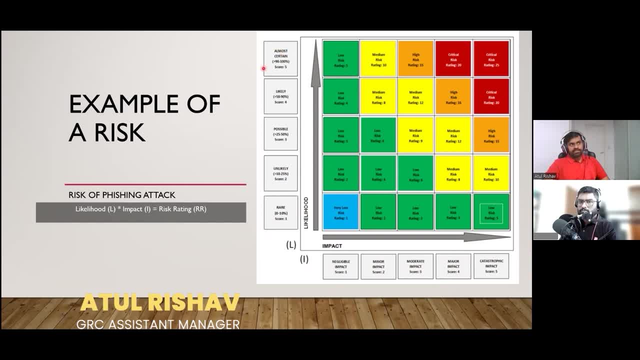 belong. i mean, which quadrant does it belongs to? so for me. belongs to, so for me. belongs to, so for me, all right. i said that it's almost all right. i said that it's almost all right. i said that it's almost certain and it's quite major, so for me. 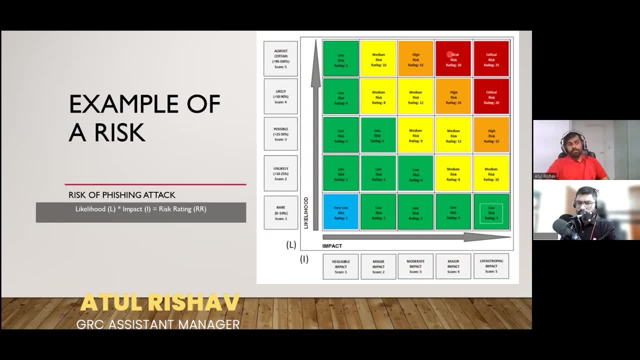 certain and it's quite major. so for me, certain and it's quite major, so for me, the risk is very critical. the risk is very critical. the risk is very critical now, now. now, when the risk becomes critical to me, when the risk becomes critical to me, when the risk becomes critical to me, i need to prioritize this risk. i need to. 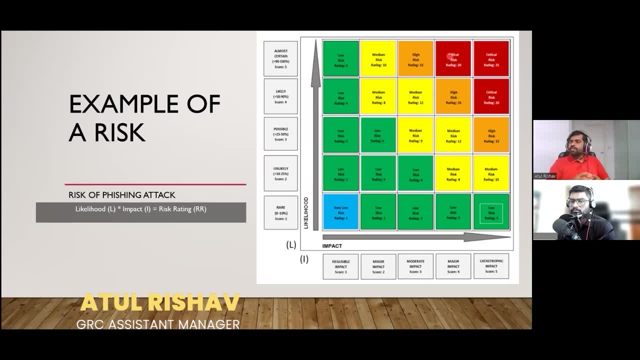 i need to prioritize this risk. i need to. i need to prioritize this risk. i need to raise this with the management to make, raise this with the management to make, raise this with the management to make sure that we have all the appropriate, sure that we have all the appropriate. 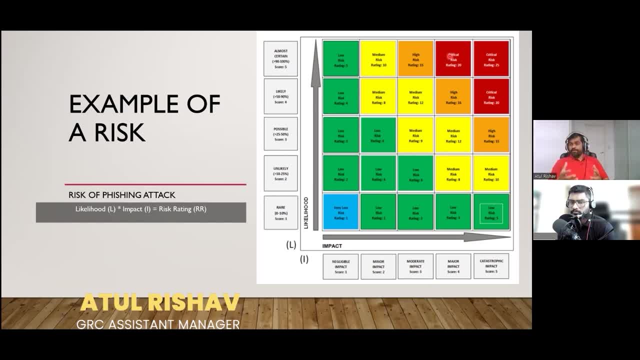 sure that we have all the appropriate controls that we need as a firm in place. controls that we need as a firm in place. controls that we need as a firm in place, right, if you don't have it already, so right, if you don't have it already so. 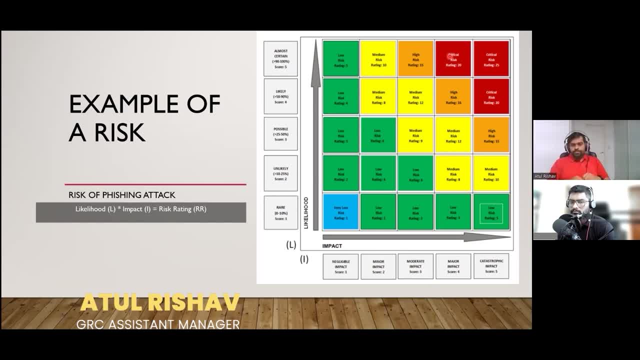 right if you don't have it already. so there could be two scenarios here: the. there could be two scenarios here, the there could be two scenarios here. the first scenario could be first scenario could be. first scenario could be. you don't have the tools at all. you. you don't have the tools at all. you, you don't have the tools at all. you don't have the expertise you need to hire. don't have the expertise you need to hire. don't have the expertise you need to hire people. you need to, you need to, you need. 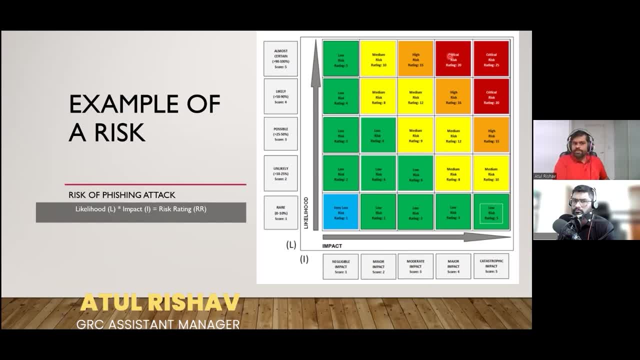 people you need to. you need to. you need people you need to. you need to. you need to onboard certain tools. to onboard certain tools. to onboard certain tools into your, into your it informant, to into your, into your it informant, to into your, into your it informant, to make sure that the phishing attacks are. 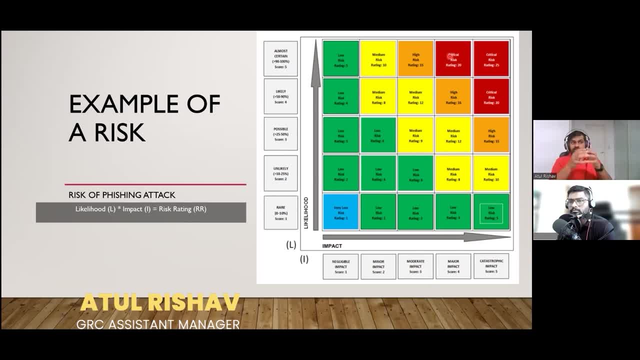 make sure that the phishing attacks are, make sure that the phishing attacks are mitigated as much as possible. right in mitigated as much as possible, right in mitigated as much as possible, right in those cases you need financial support. those cases you need financial support. those cases you need financial support from the organization. and that's when 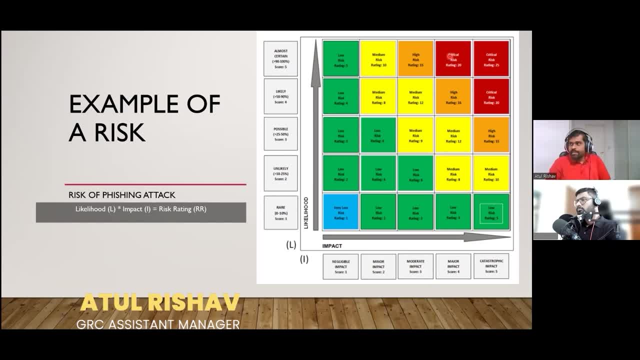 from the organization and that's when from the organization and that's when you hold you, hold you hold thousand, you hold, you, hold, you, hold, thousand you hold, you hold, you hold thousand dollars worth of data and to save that- dollars worth of data and to save that. 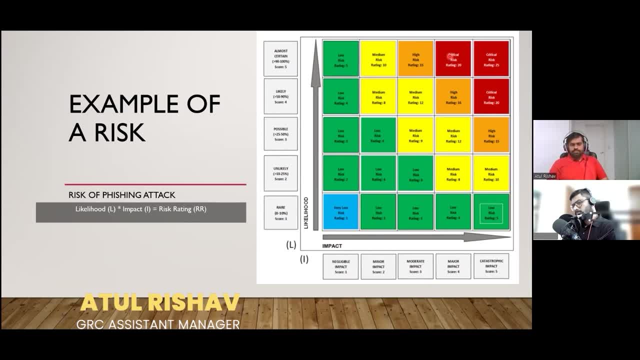 dollars worth of data and to save that? there's this, uh uh, another, you know. there's this, uh uh, another, you know. there's this, uh uh, another, you know. let's throw another hundred hundred. let's throw another hundred hundred. let's throw another hundred hundred twenty dollars, which would, which would. 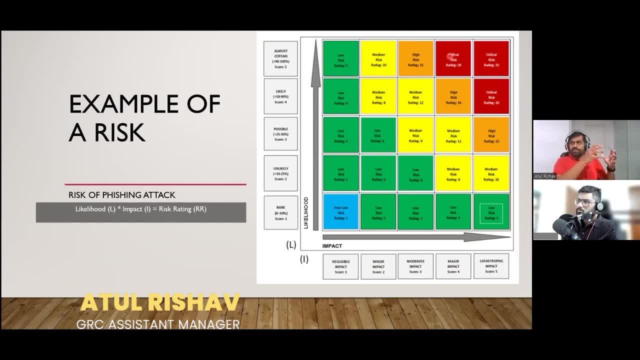 twenty dollars, which would, which would, twenty dollars, which would, which would, which would cost you to save that thousand, which would cost you to save that thousand, which would cost you to save that thousand. dollars of data, right, so that. dollars of data, right, so that dollars of data, right. so that makes sense as an organization to me. 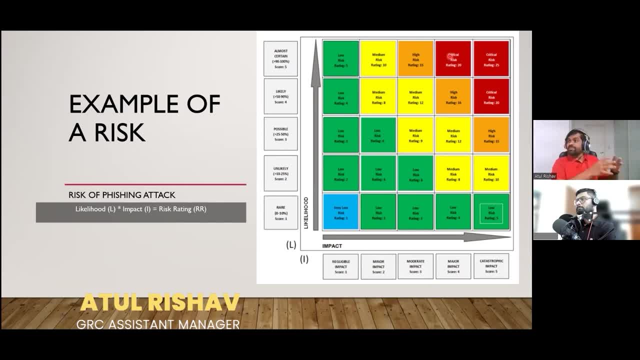 makes sense as an organization to me, makes sense as an organization to me that let's, let's spend some money and that let's, let's spend some money and that let's, let's spend some money and save that data, because that's really save that data, because that's really 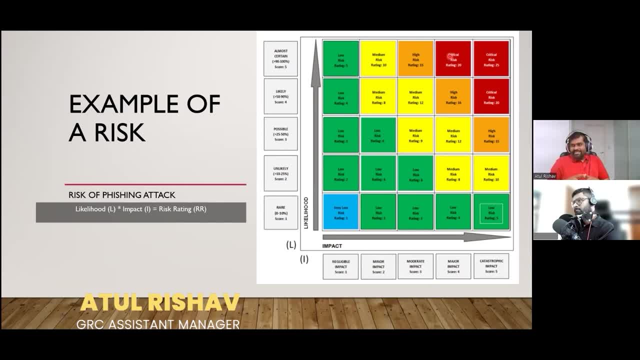 save that data, because that's really critical to me right now, in certain critical to me right now, in certain critical to me right now, in certain cases, cases, cases, if, if, if the mechanism or the money that you are, the mechanism or the money that you are, the mechanism or the money that you are investing to actually save, 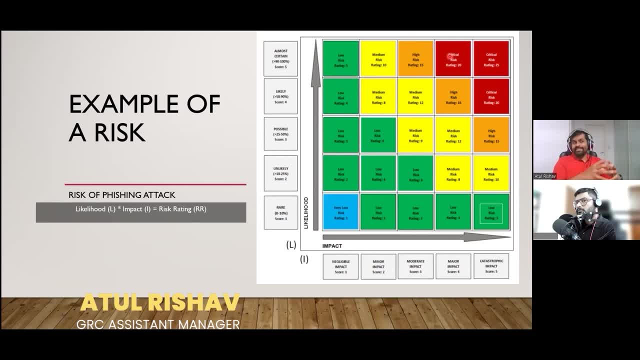 investing to actually save. investing to actually save. safeguard that data. safeguard that data. safeguard that data surpasses that. it doesn't make sense to surpasses that. it doesn't make sense to surpasses that. it doesn't make sense to me as a firm to actually save that data. 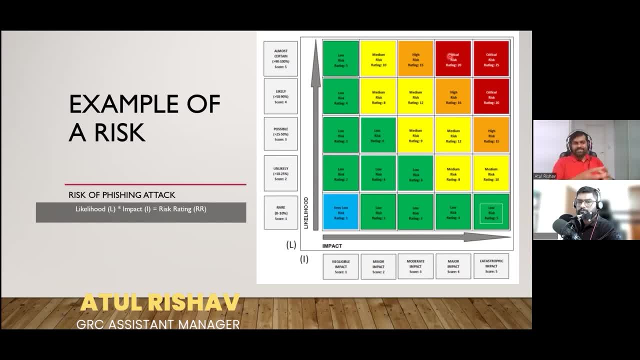 me as a firm to actually save that data. me as a firm to actually save that data. right, so say that. if i have a thousand right, so say that. if i have a thousand right, so say that. if i have a thousand dollars asset and to safeguard that i. 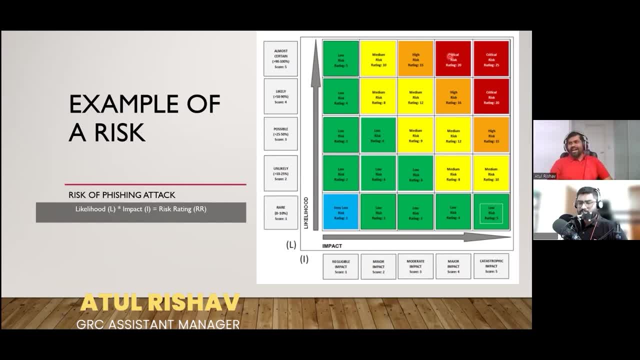 dollars asset and to safeguard that i dollars asset and to safeguard that i need to throw another three thousand, need to throw another three thousand. need to throw another three thousand dollars might as well. thousand dollars might as well. thousand dollars might as well. thousand dollar. data right, so it doesn't. 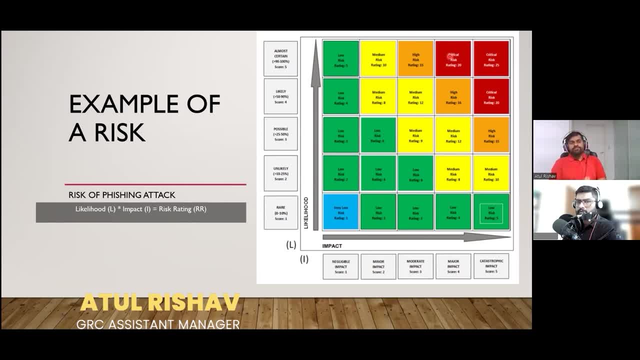 thousand dollar data- right, so it doesn't. thousand dollar data, right, so it doesn't make sense. make sense: make sense to me as a business, right? so now that we to me as a business, right, so now that we to me as a business, right so now that we have identified the data, is i mean the 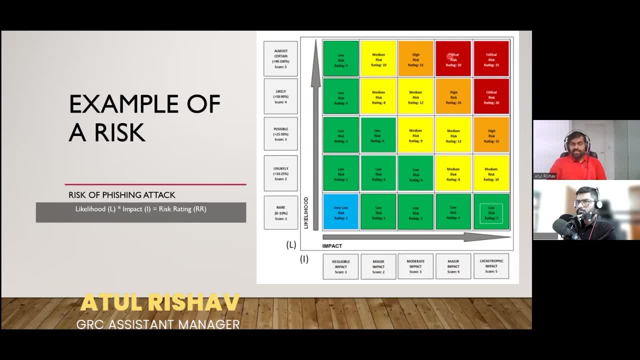 have identified the data is, i mean the have identified the data is, i mean the risk is really critical. we need to make risk is really critical. we need to make risk is really critical. we need to make sure that this gets highlighted. sure that this gets highlighted, sure that this gets highlighted with the board, with the management and 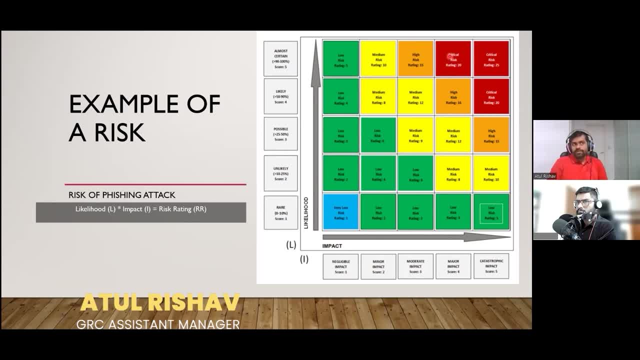 with the board with the management and with the board with the management, and make sure that we take all the make sure that we take all the make sure that we take all the appropriate controls and all the appropriate controls and all the appropriate controls and all the appropriate measures to reduce that to. 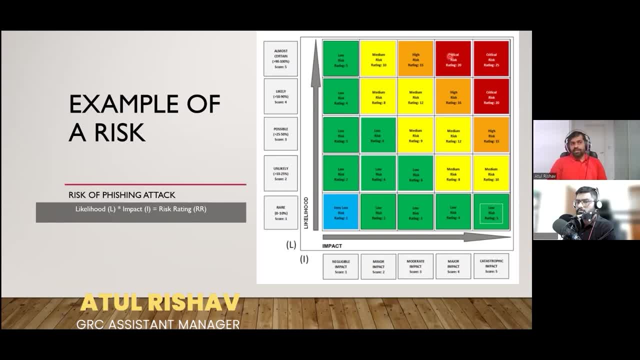 appropriate measures to reduce that to appropriate measures to reduce that to an acceptable level for me, as i said, an acceptable level for me, as i said, an acceptable level for me, as i said for me, since i'm operating into a highly, for me, since i'm operating into a highly. 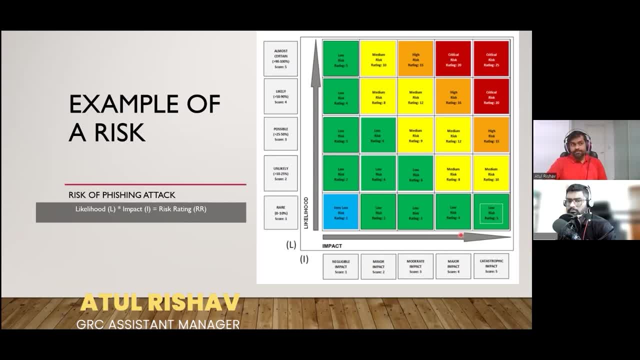 for me, since i'm operating into a highly regulated industry- the regulated industry, the regulated industry, the- the acceptable level for me is low. the acceptable level for me is low. the acceptable level for me is low. right, this is, this is. this is what i right. this is this is this is what i.